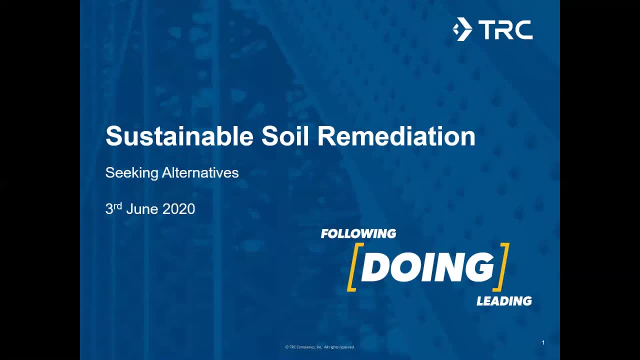 into the background of the traditional dig and dump method, why it's been a preferred method for many years, its negative impacts and how we as consultants are going to be interventionist. as얼 consultants and remediation contractors could look into more innovative. 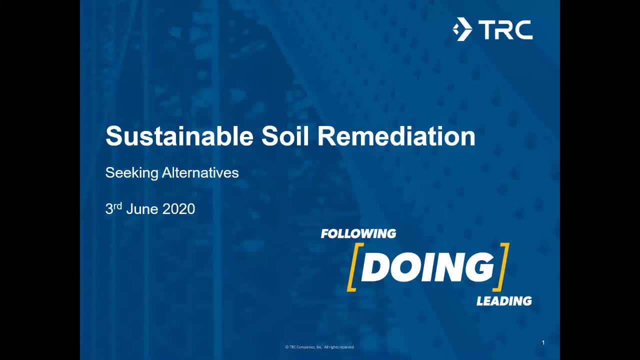 methods of remediation that can effectively remediate the site whilst having minimal environmental, social and economic impacts. I would like to just stress that the purpose of this presentation is to promote discussion on more sustainable remediation options. It's not about what's. 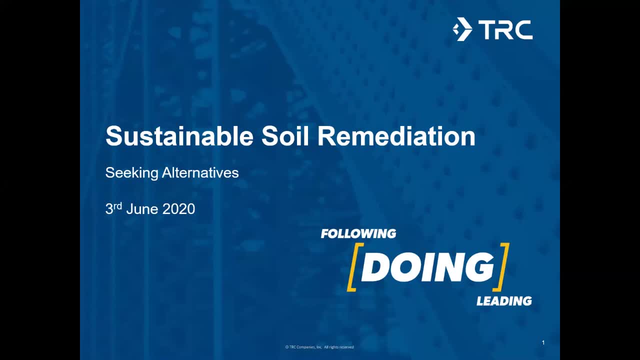 the right and wrong way to remediate contaminated land. Everyone has their own opinion. Every site is different, So thank you for your time and I hope that you'll have a good discussion. Thank you for having me. Thank you, Thank you. 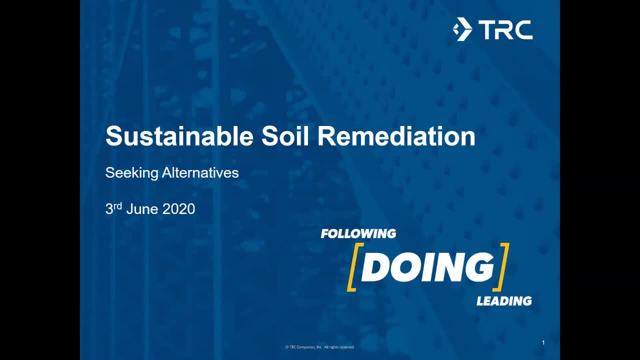 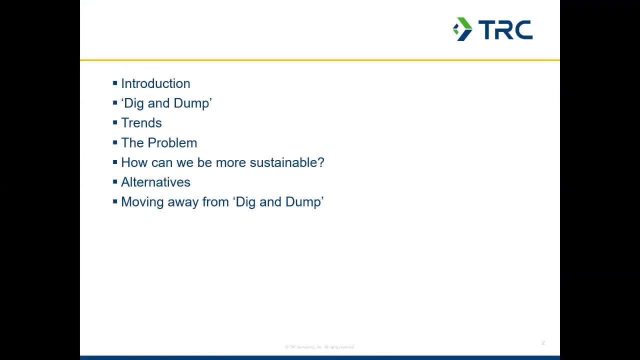 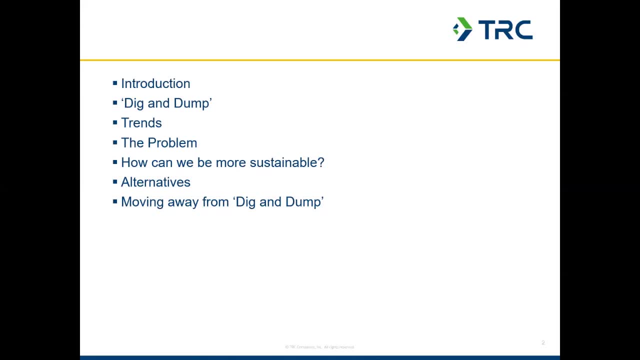 introduction into remediation, the reasons for it, and I'll then provide a background on dig and dump and why it's been seen as the preferred method for a lot of clients. Then I'm gonna follow that up with the trends in dig and dump and then I'm going to talk about some of the problems that dig and dump has and the negative. 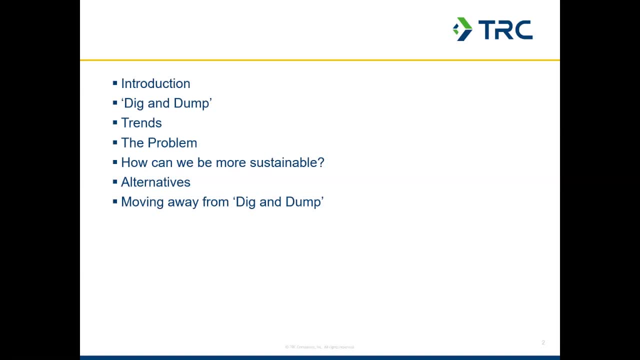 impacts it has on the environment. Then I'm finally going to talk about some alternatives we should be considering to replace this method of remediation and finally discuss how we can work with clients, see the benefits of moving away from dig and dump to use more innovative and 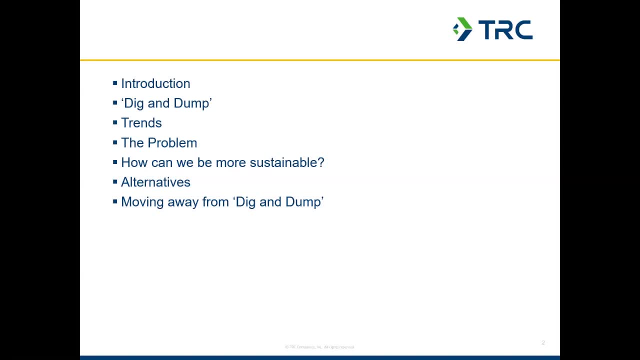 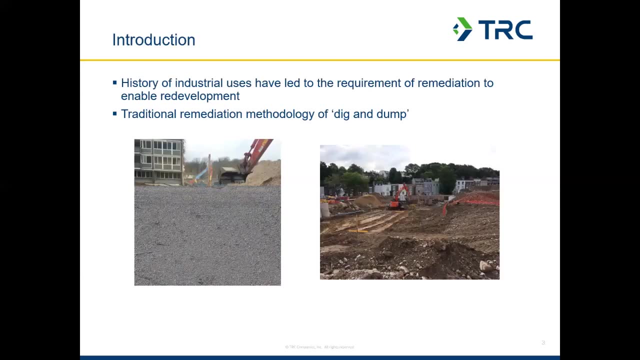 sustainable methods of remediation. So we've got a history of heavy industrial use that has led to the requirement for remediation in order to be able to redevelop, and the traditional method of remediation on sites have largely involved dig and dump can involve excavating large quantities of contaminated soils and disposing it. 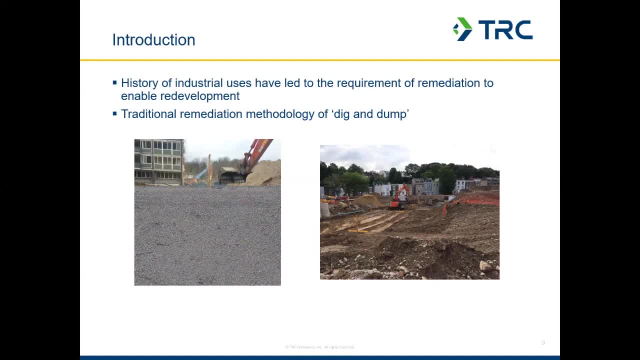 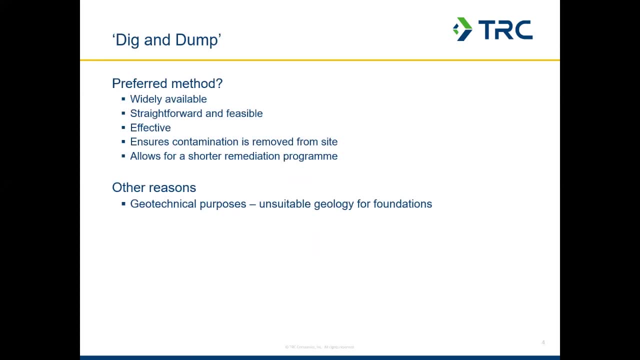 off-site at various landfills, soil treatment facilities or reclamation facilities. A lot of clients tend to opt for this method of remediation rather than considering other options, so I'm going to talk a bit about why clients might prefer this method. Dig and dump has. 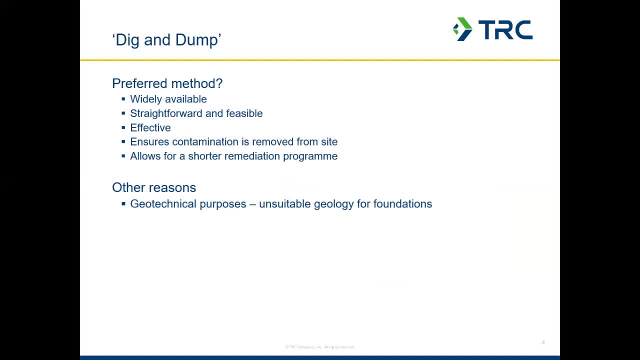 seemed to be one of the most popular methods of remediation in the world and is seen as a widely available method of remediation. It's generally seen as being very straightforward and feasible on the majority of sites. It's seen as an effective and quick fix solution to contaminated land. It ensures 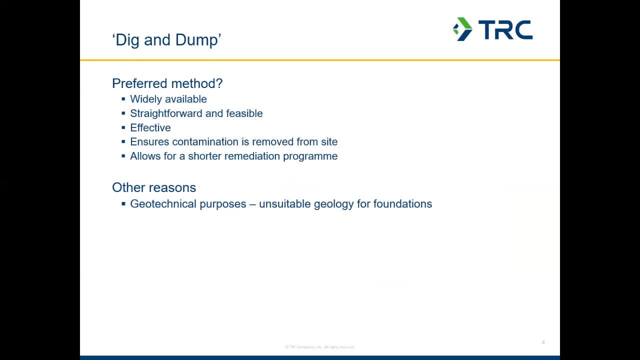 contamination is removed from site, and one of the greatest benefits of dig and dump, as seen by clients, is that it allows for a shorter remediation program, which in a lot of cases, is what the client needs. In my experience, having worked for a lot of developer clients, particularly in the 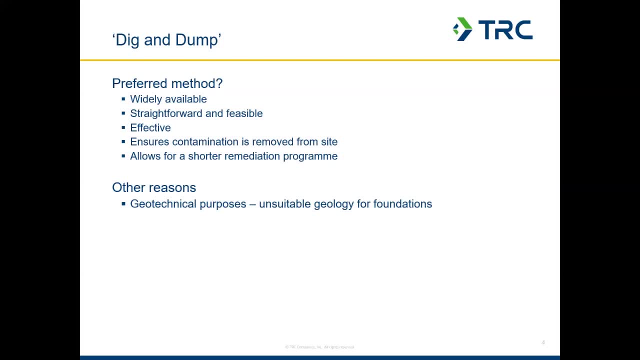 commercial sector. they tend to have very short programs and so this method of remediation suits them well, and, as a result, they're less likely to consider any other option. Other, more innovative remediation options may involve further assessment and design, which can lead to additional costs for the client and potentially require more time, and therefore it lacks. 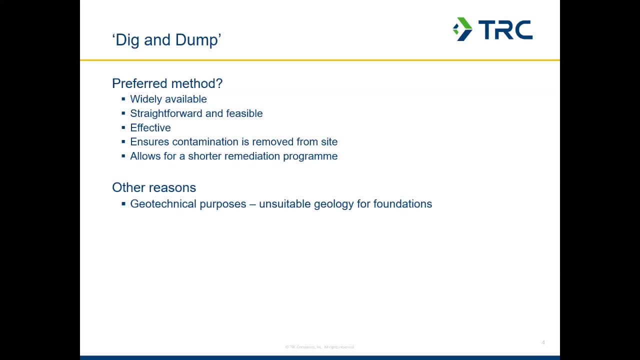 appeal. There are other reasons besides environmental, where you may be looking to excavate large quantities of soils for removal, and an example of this is for geotechnical purposes. There are times where a site may not have the ground conditions or geology suitable for founding on and, as a result, that may 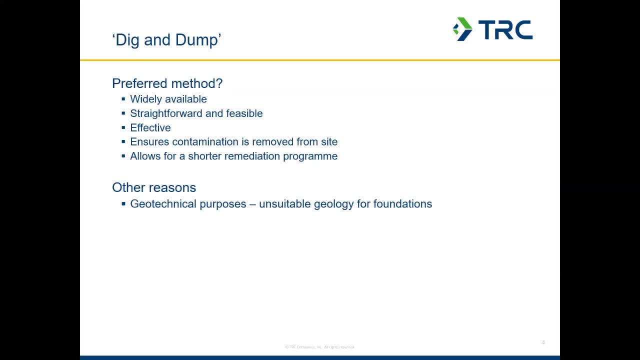 lead to its removal. This could include variable made ground or very soft layers on a site such as peat, which could which would be deemed unsuitable for foundations. Clients may see the removal of this material as the most straightforward way of dealing with unsuitable ground conditions, rather than consider options such as ground. 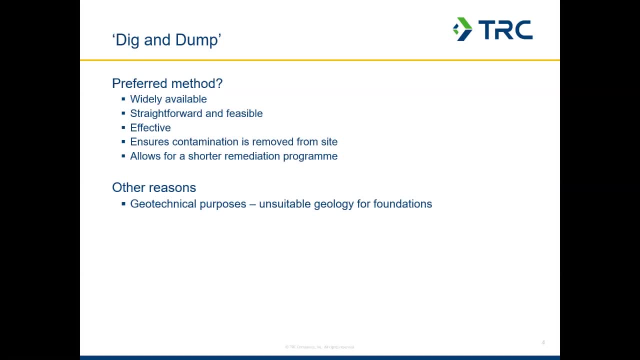 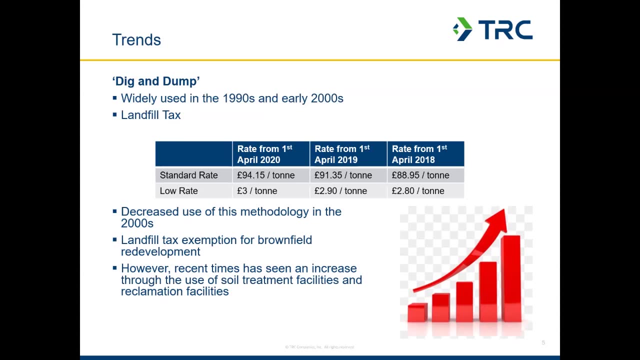 improvement. So moving on to the trends seen for dig and dump. So, moving on to the trends seen for dig and dump, This was something that was widely used in the 1990s and early 2000s. However, the implementation of landfill tax in the late 1990s and its subsequent 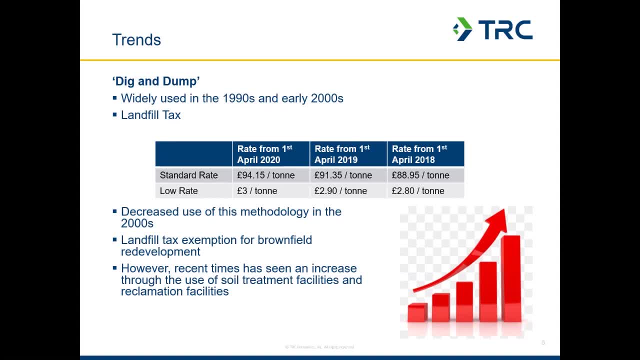 escalation, whose aim was to minimize waste disposal and to encourage alternative means dealing with waste through options such as recycling, led to a decrease in this methodology in the 2000s, Although there was landfill tax. there was also landfill tax in the 1990s. 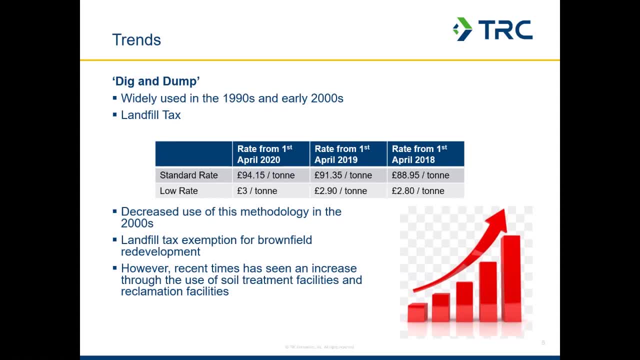 Although there was landfill tax, there was also landfill tax in the 1990s. There was also landfill tax exemption for ground field development, which was a government incentive to encourage remediation of ground field land, yet in a sense promoted the use of dig and dump as the means for remediation. 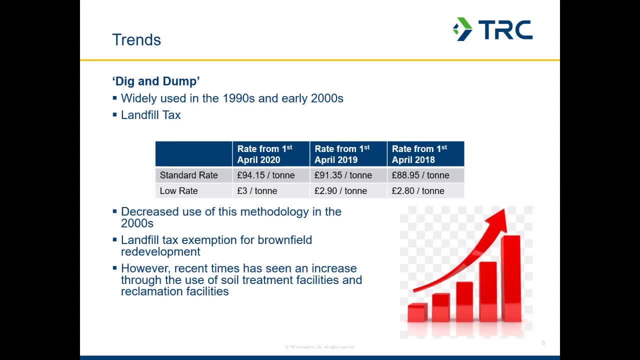 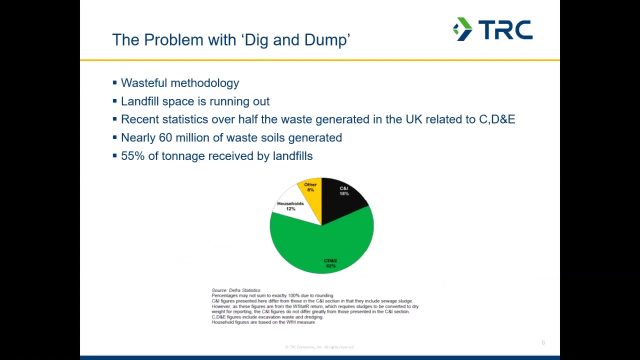 Also, in recent times, with the introduction of soil treatment facilities and reclamation facilities, there has been an uptick in excavating and removal of contaminated soils instead of considering other remediation options. However, there are multiple problems with the dig and dump methodology. Firstly, it is considered to be a very wasteful methodology with landfill space fast running. 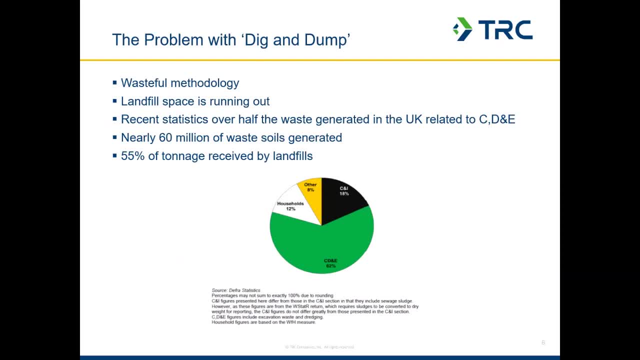 out and, with the rise of landfill tax, more consultants are looking at alternative ways to remediate. Government statistics show that over half the waste generated by landfill is being collected by the UK is related to construction, demolition and excavation, with the most recently available information showing that in 2016, nearly 60 million tonnes of waste soils were. 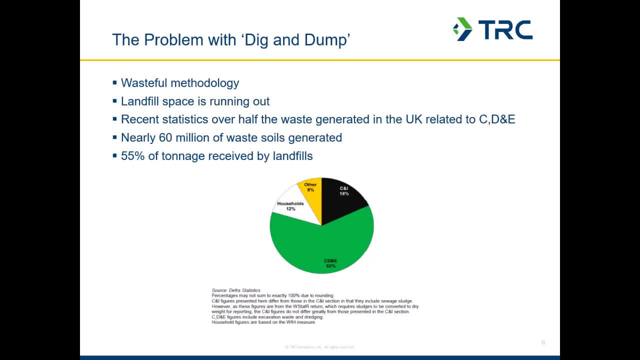 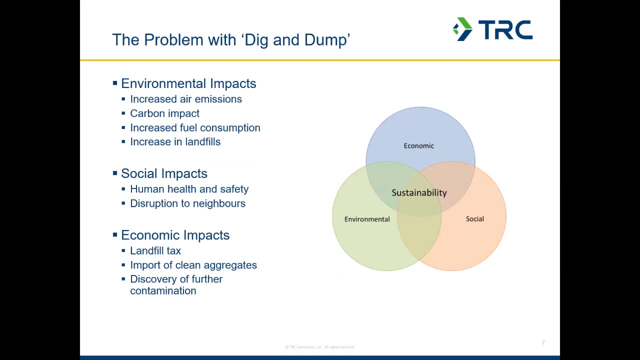 generated, and soils make up to 55% of the tonnage received by landfills. So just continuing on with discussing the problem with dig and dump. Whilst remediation, which allows for the reuse and redevelopment of previously contaminated land, may be seen as sustainable practice, to get to that point will result in environmental 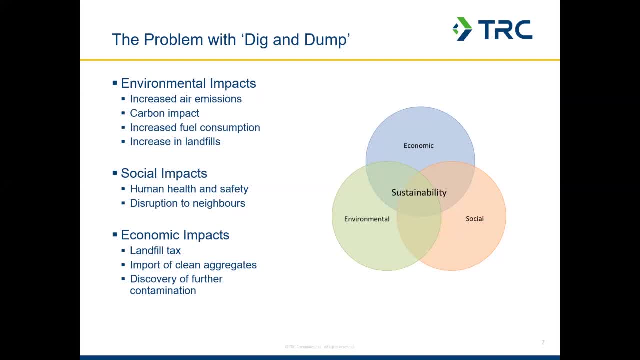 social and economic impacts. It is therefore important that the remediation methodology selected does not cause a greater negative impact than the contamination you are trying to remediate. There are a number of environmental, social and economic impacts associated with dig and dump. We are starting with the environmental impacts. you have got the haulage of soils from sites. 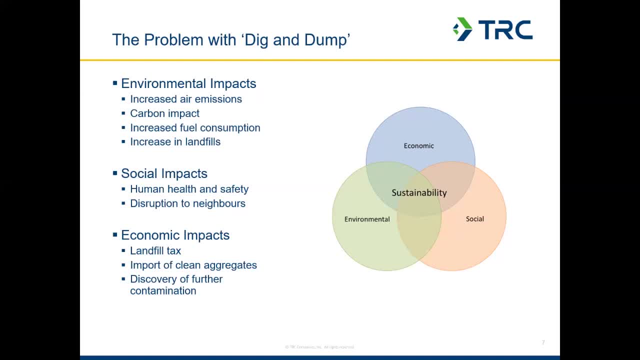 to landfill or soil treatment facilities, which will lead to increased fuel consumption, increased carbon impact, air emissions and noise pollution through the trucks running up and down the roads from between the site and various facilities. The soils will likely get disposed of at a landfill, which 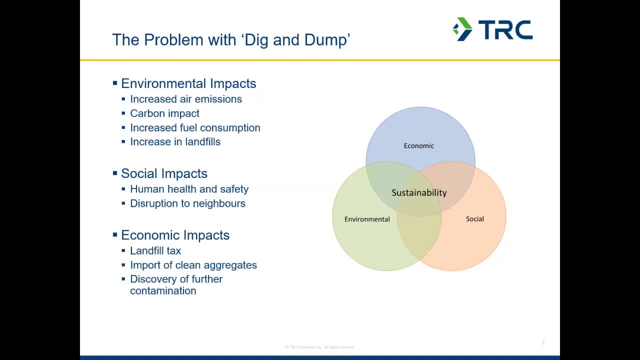 isn't ideal. It is likely that once you have excavated and removed the contamination, you will need to backfill and reinstate the excavation using clean imported materials. This again will require significant haulage of material, which once again leads to increased fuel consumption. air emissions, noise pollution, carbon impact. 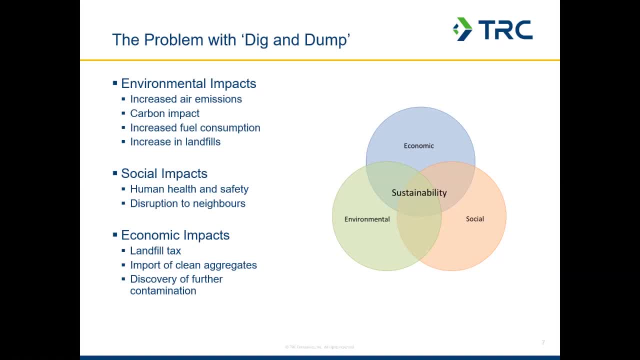 Social impacts of dig and dump will include health and safety aspects, such as the use of heavy plant on site, Exposure to contaminants and heavy vehicle movements on site Albeit short term, there could also be disruption to neighbours through the increased site activity, heavier traffic, dust and noise generated. 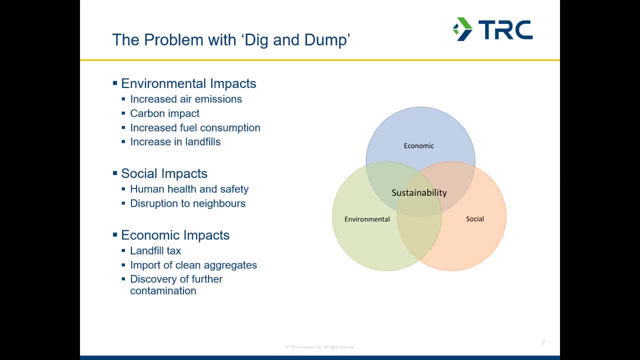 Some of the economic impacts would include the costs of undertaking the work, so landfill tax and disposal costs, costs of mobilisation and plant use. The potential for import. The potential for import. The potential for import of clean aggregates, if required, will also be costly and the potential. 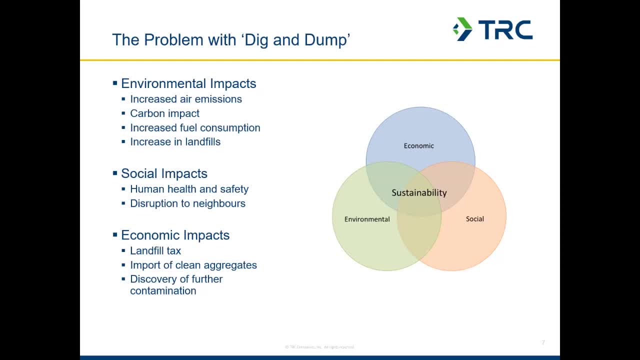 for discovering further contamination could lead to increased remediation costs, as further excavation and removal of material may be required. All three aspects need to be considered in any remedial design in order to achieve a sustainable outcome. A couple of other points to consider when looking at environmental impacts of this method is: 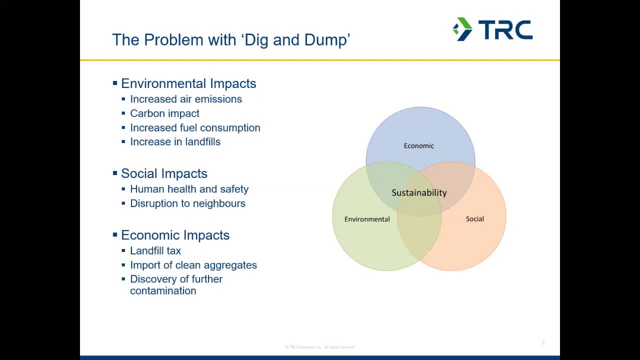 that, although you are removing contamination from one site, you are merely relocating the problem, not solving it, by moving the contaminated soils from one location to another location, albeit one that has more controls in place, Whilst the presence of soil treatment facilities and reclamation facilities have led to less. 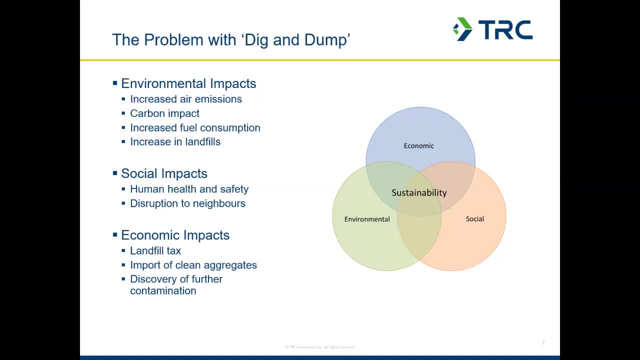 disposal of contaminated soils to landfill, you still have to contend with the amount of soil haulage there will be in order to treat the soil. Soil haulage is an important part of the process. It is not just a matter of time before the material is transported to these facilities. 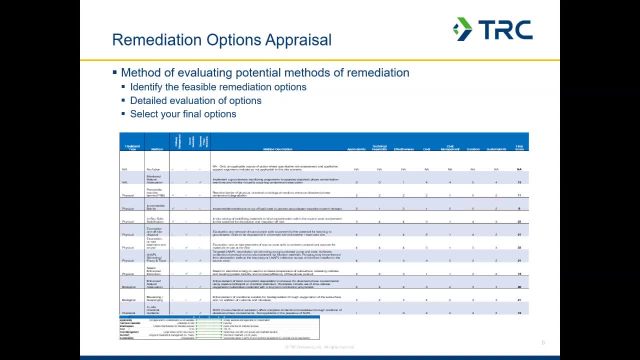 In an ideal situation, a remediation options appraisal will be undertaken to aid selection of the most appropriate method. I have put up an example on this slide. However, please note there are other ways an appraisal can be undertaken. This is just one way of doing it. 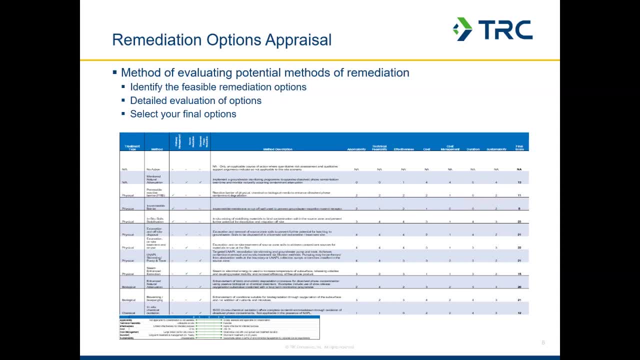 A remediation options appraisal is undertaken through attraction of the material to the tiered approach, So tier one. you identify the feasible remediation options for the site. This will consider the objectives and criteria set for the site. Important to consider things like the site setting practicality, accessibility of the site, current site status, stakeholder. 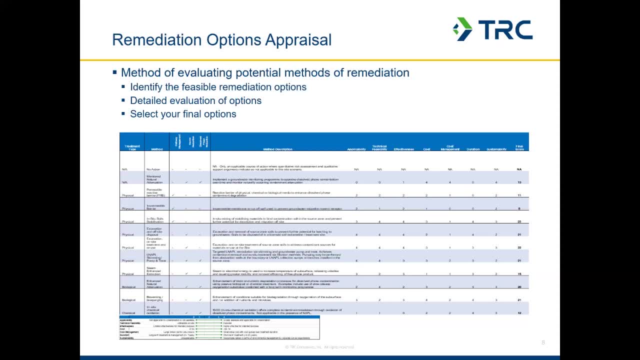 views such as regulators and site owners and neighbouring properties. You then have the second tier, where you evaluate each of the shortlisted options you determine in tier one. You could produce a matrix similar to the one presented here and assess each option based on a point scoring system. Things to assess would include how applicable is. 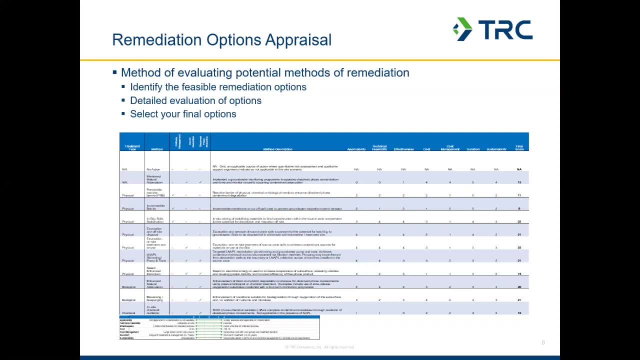 the method. how feasible is this method on the site? how effective is this method? what are the cost implications? what are the cost management such as the method have a large initial cost, or is it a small initial cost, with the cost spread over treatment duration, the duration of the remediation itself? so does it require long-term 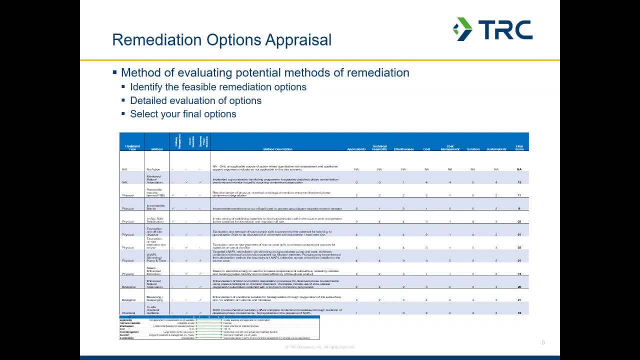 treatment and management, or is it a short-term solution? and finally, how sustainable is this method? The final tier is to select options that will deal with the site as a whole, So it may lead to consideration of whether you can combine multiple options and, if possible, 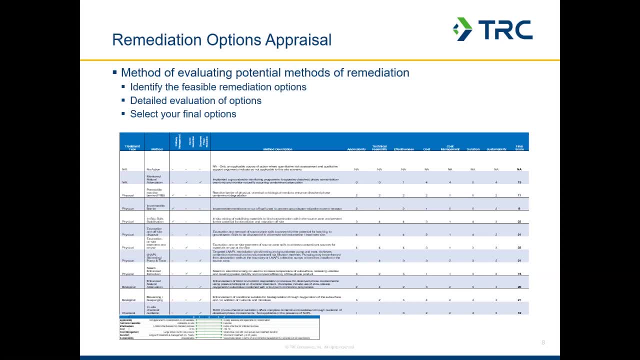 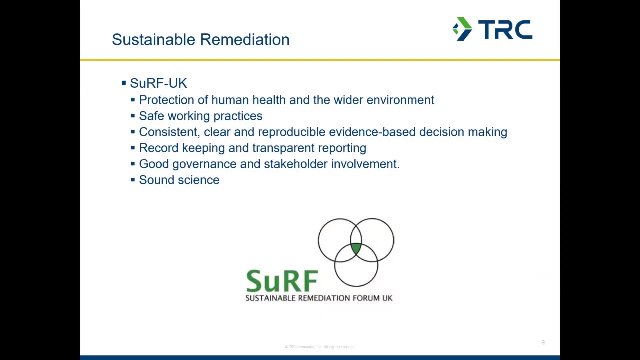 the practicality of combining multiple options. This may then lead you to have to reassess and revisit previous tiers. As mentioned previously, remediation options appraisals do vary and no one way is correct. The contaminated land sector is always looking at new ways to improve remediation practices. 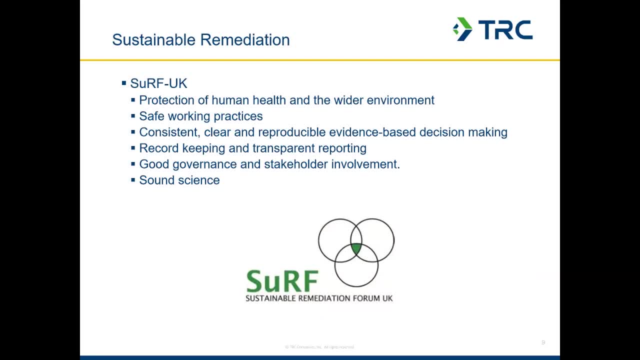 Presently, one of the things that is strongly considered when selecting remediation methods is how sustainable it is. Unfortunately, even with a remediation options appraisal, a lot of the time clients' objectives are driven by time and costs and, as a result, we are often 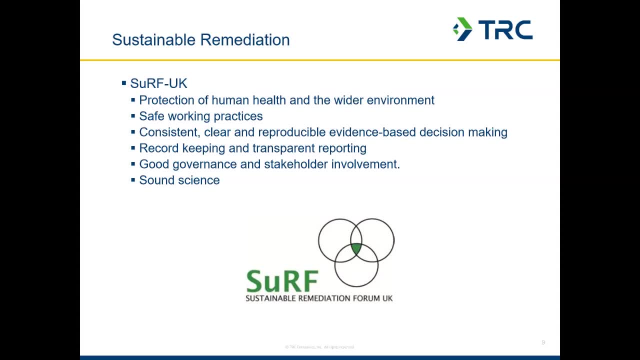 left with one option, and that is excavation and removal of soils from site. There are initiatives out there, such as the UK Sustainability Remediation Forum, which was set up in the late 2000s. It was developed to aid a balanced decision-making process in terms of sustainable remediation. 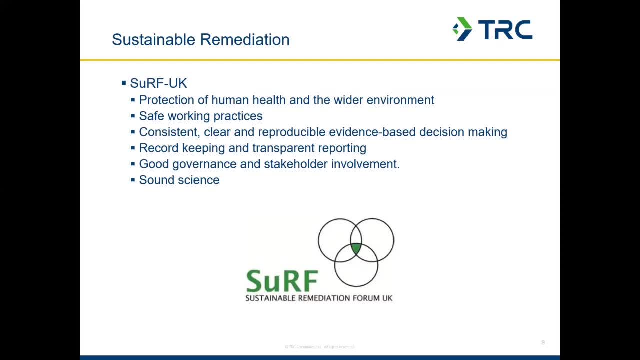 This initiative looks to encourage the consideration of sustainability associated with potential remediation early on in the site's redevelopment process. It targets not just those who produce the remediation options, appraisals or strategies, but a wide range of stakeholders including the site owners, consultants, remediation contractors, the local community regulators. 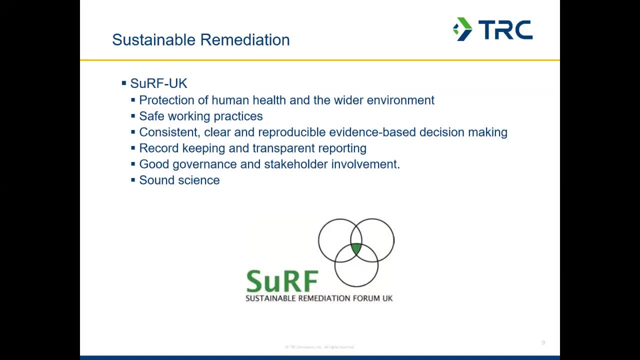 town planners and local government. The project is to encourage the consideration of sustainability associated with potential remediation early on in the site's redevelopment process. It targets not just those who produce the remediation options, appraisals or strategies, but a wide range of stakeholders, including 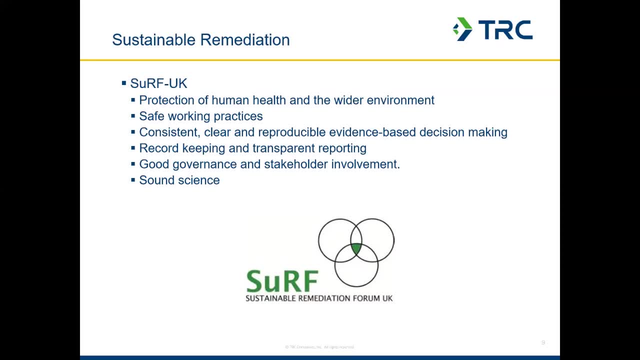 the site owners, consultants, remediation contractors and local government. The framework identifies six key principles, so protection of human health and the wider environment. for example, it should remove unacceptable risks to human health and protect the wider environment now and in the future for the agreed land use and give due consideration. 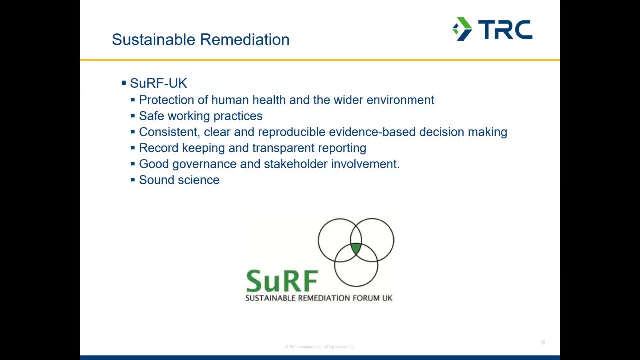 to the costs, benefits, effectiveness, durability and technical feasibility of available options. The framework identifies six key principles, so protection of human health and the wider community, for example, and it should eliminateWith End ung, you've grown amongst the staff who have continued to work in RDAS. The framework also outlines which principle 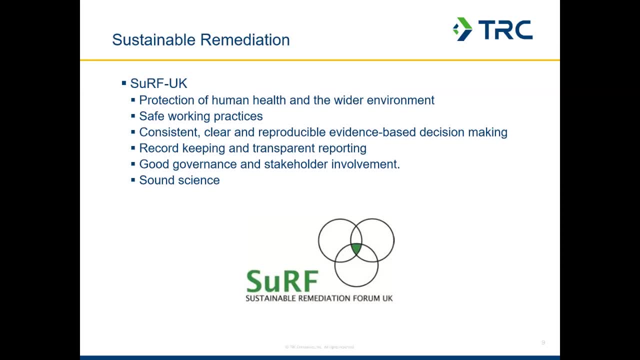 many of us have chosen to Star. well, The framework identifies six key principles, so potential relief items, частly related to our current role in the system, Are responsive. facing what are the doctor's myself is what I feel priorities were use. 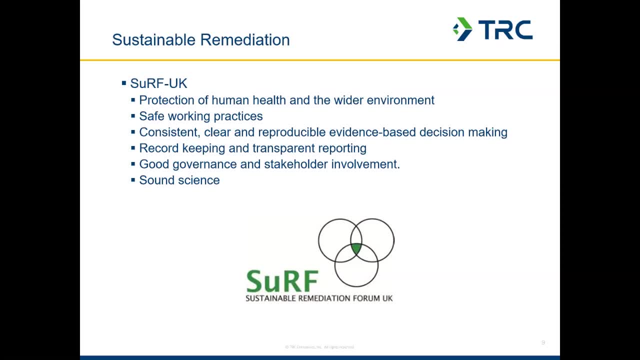 of what I hope be wearable and helpful for myself. a SME souvenir that would bring a change in occasions, make the decision more Bearable to the patient, to touch upon and анти the actual needs. The framework conveys the individual's readability, the most general importance to those who dichorte. 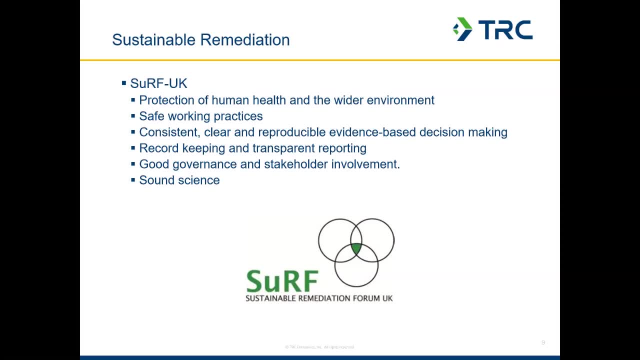 records kept showing the supporting data used and assumptions made, which demonstrates to interested parties that a sustainable solution has been adopted. Good governance and stakeholder involvement: so it's important to consider stakeholders views and allow them to participate, which will contribute to the decision-making process and sound science. so all 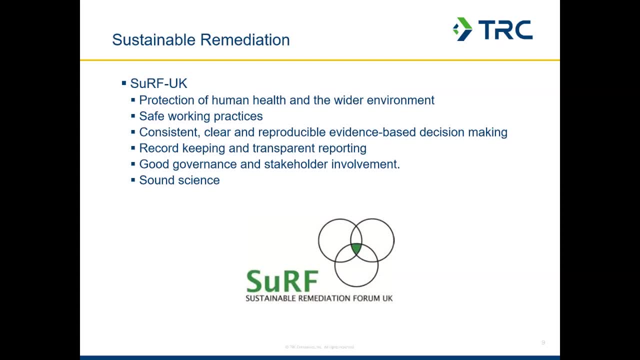 decisions should be made on accurate and reliable data and also based upon the best available information. So SURF UK has 15 indicators- so five social, five economic and five environmental- that can be utilised for your sustainability assessment when it's undertaking remediation options, appraisal As 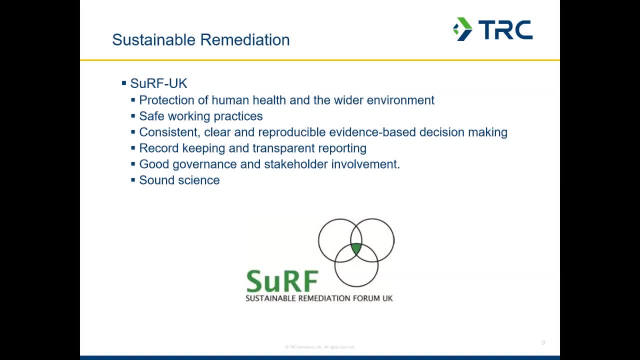 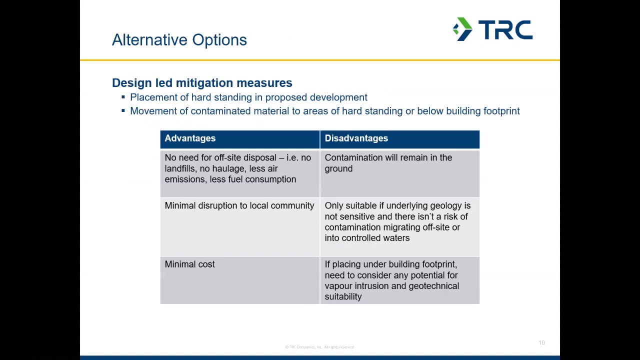 mentioned, it is very important, where possible, to engage with clients early on and inform them of things they need to consider, such as remediation, when they are developing their programme. by doing this, you stand a better chance of being able to consider and select a remediation option that does consider sustainability. And so, as mentioned, 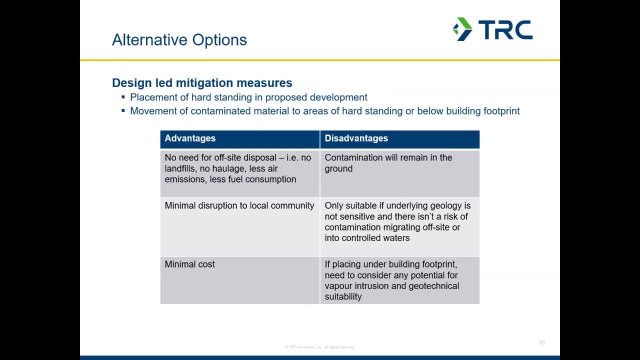 previously, it's important to look for other ways to remediate, which strongly considers sustainability. I'm now going to briefly go through some alternatives that can be considered when looking to remediate contaminated sites and talk a bit about the advantages and disadvantages of each. The first option is to determine whether there can be any design led. 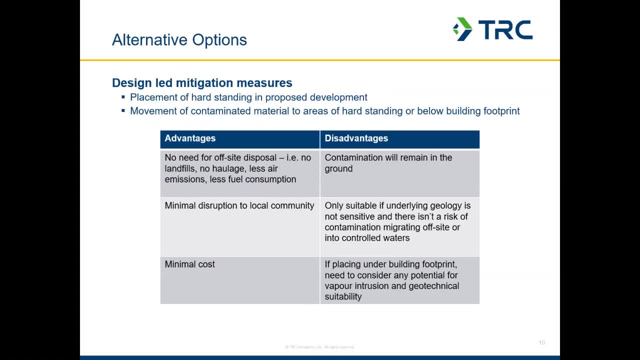 mitigation measures that can be adopted at the site. This might include the placement of hard standing at the proposed development, so it works well for commercial type developments where you have service yards and minimal soft landscaped areas, and the material could also potentially be moved to other areas. 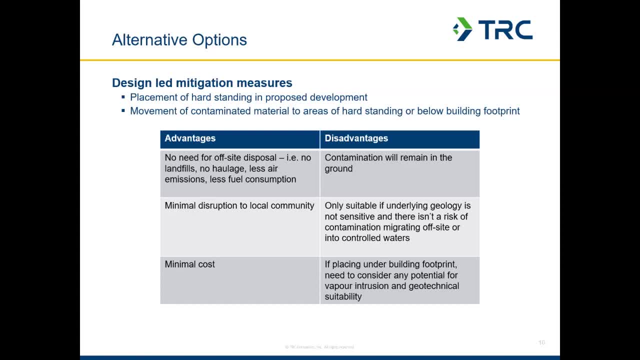 of the proposed development where hard standing will be placed or below the proposed building footprints. The benefits of this would include removing the need for any off-site disposal, thus not requiring landfills, and, as a result, there will be no haulage, which will then lead to less air. 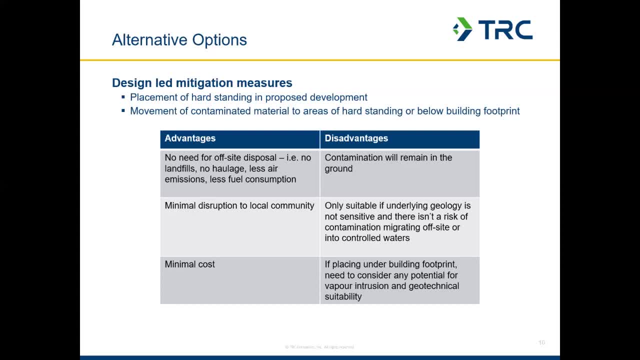 emissions: less fuel consumption, less noise, less dust generation. This method would also lead to minimal- or, as mentioned, would lead to minimal- disruption to the local community and generally will be considered a safer method, as there will be a decrease in lorries entering. 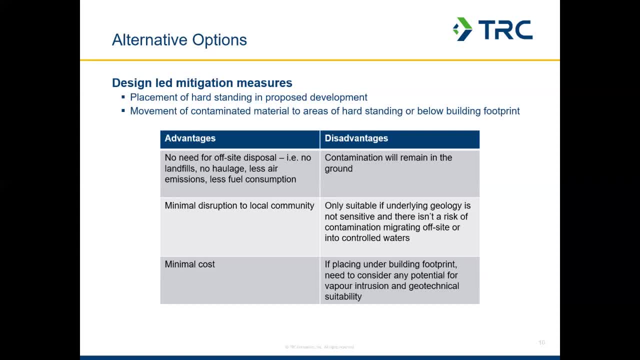 and leaving the site. There will also be less cost involved in this method, as you will be removing any potential for disposal costs and haulage of material. However, when looking at design-led mitigation measures, there are things that need to be considered, which include: 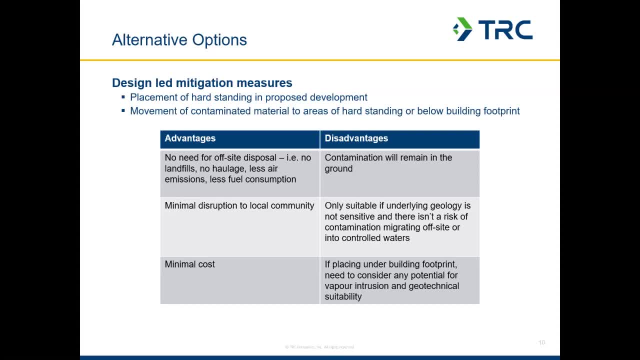 a fact that contamination will remain in the ground and this should be recorded for any future potential sale of the site and any other future redevelopment. This method would also only really be suitable if there are no other receptors that would be at risk, such as controlled waters and migration off-site to neighbouring properties. So it wouldn't. 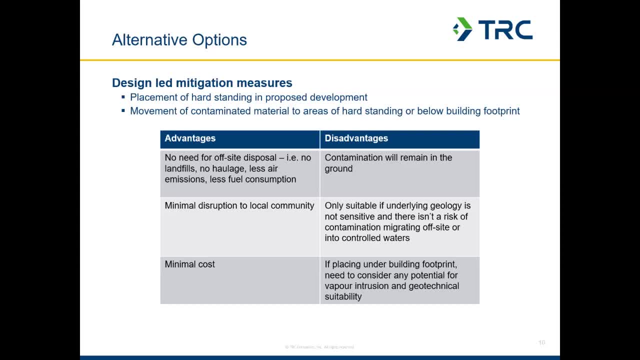 work on sites that have sensitive aquifers underlying it. It would only be suitable for sites that have low permeability soils, which would limit any migration off-site. Also, if you are placing any potentially contaminated soils underneath the footprint of a building, it is important to make sure that there are no risks from. 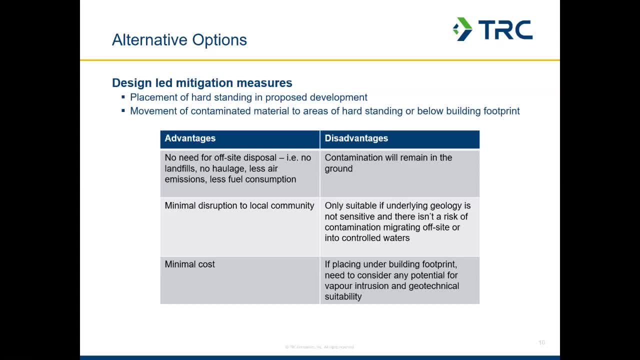 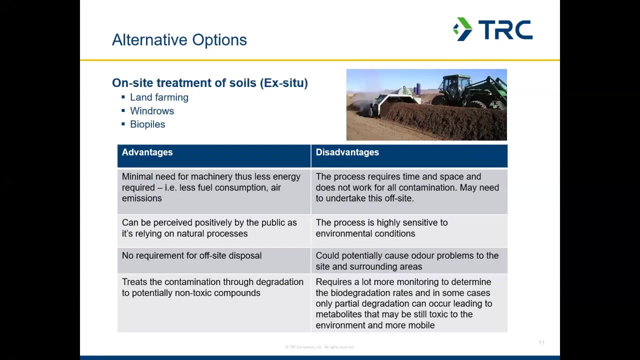 vapour intrusion in the proposed building, particularly if there is hydrocarbon contamination present, and also it is important to consider the geotechnical suitability of the material that you're using for foundations. On-site treatment soils could also be considered. Examples of this would be things like land farming. 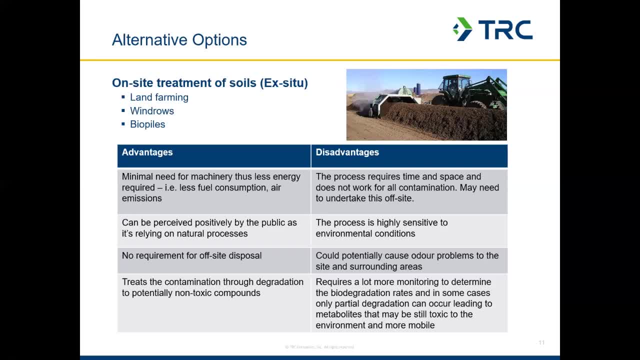 wind rows for hydrocarbon contaminated soils, where you'll excavate the contaminated soil and place it on the ground surface, add nutrients, minerals and moisture, and turning it regularly to promote microbial activity, thus aiding the degradation of the hydrocarbon contamination to an acceptable level. 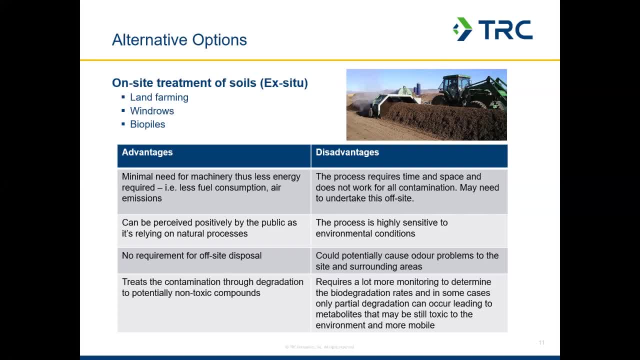 before placing the soils back into the ground. Biopiles is another method whereby you can excavate the contaminated soils and place it in a shaped pile and aerate it using something like a vacuum pump. The vapours can be treated using granulated activated carbon to reduce 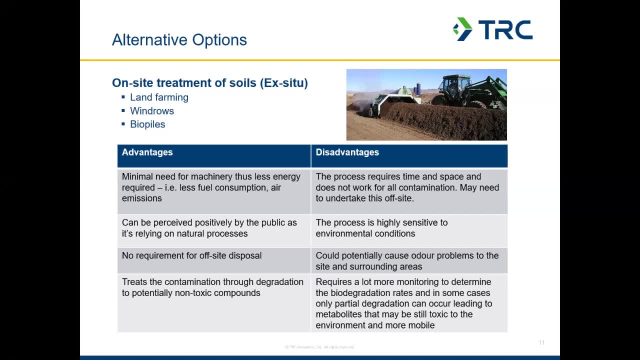 any emissions. The benefits of on-site treatment of soil includes minimal requirements for extensive amounts of equipment machinery. therefore, less energy is required, so less fuel consumption, air emissions, and it could be perceived positively by the public because it's a method that 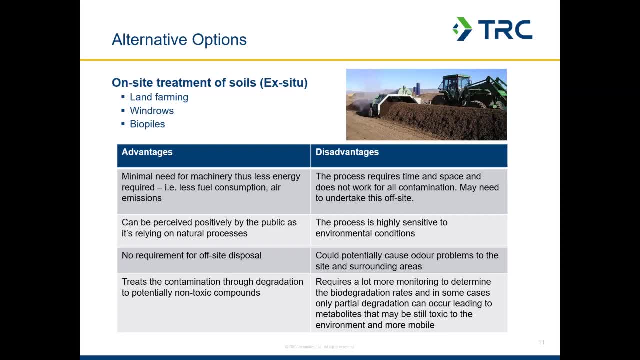 relies on natural processes only. There's no requirement for any off-site disposal. so say, if you have an off-site disposal, you can use a vacuum pump. This is effective in the record of every 1,200 debris at individual dafür, and public management should only consider. 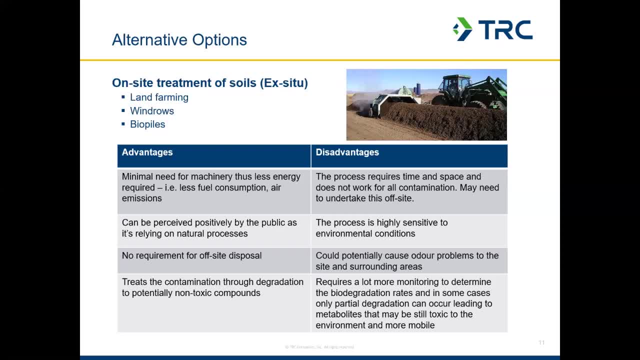 using a drip flask. You windows need to be falling as well. Ideally, the dry ground will collect all of the debris so it can Disclosure and reorganise the soil in a manner that is consistent with the soil content may end up having to carry this out off site, which could then again lead to haulage costs. 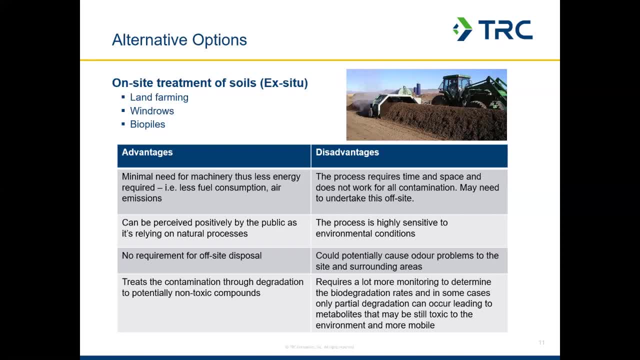 which isn't ideal because again it could lead to more traffic, again more air emissions, more fuel consumption. The process is also highly sensitive to environmental conditions of the site. it can also potentially cause odour problems to both the site and surrounding areas, so odour. 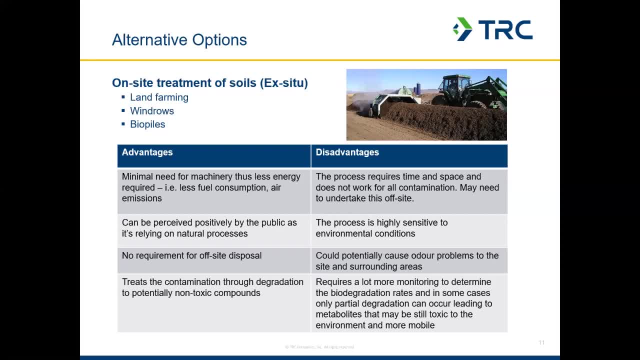 control measures will need to be considered, and also it requires more monitoring on site, which could lead to increased costs, to determine whether the process is happening and at what rate, and in some cases, there may be only partial degradation of the compound, leading to metabolites that may still be toxic to the environment and more mobile, leading to potential off-site migration. 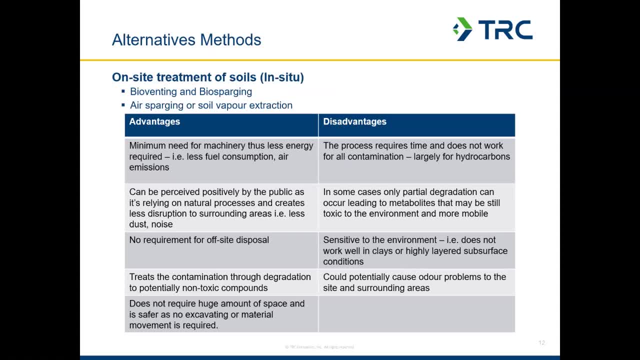 Again, you can also consider other on-site treatments of soils that don't require any kind of excavation, so soils that just remain in situ. So things like biosparging and air sparging. So biosparging utilises microorganisms to help biodegrade contaminants. 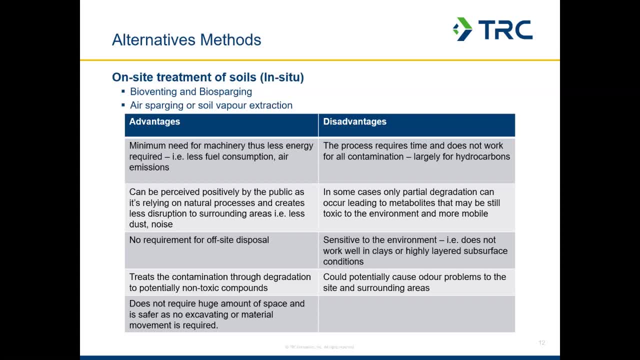 Air and nutrients are injected to aid the microorganism activity in breaking down hydrocarbon carbon. In the case of biodegradable compounds, an air sparging or soil vapour extraction involves injecting air into the soil where air bubbles are formed and travel through the contamination. 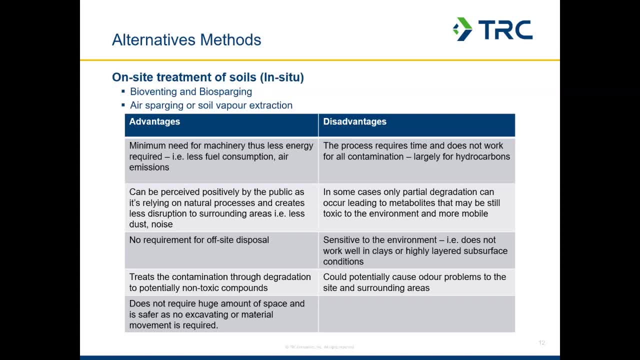 in and above the groundwater. These bubbles volatilise contamination and, in stored vacuum extraction points, extract the vapours utilising a soil vapour extraction system. The benefits of in situ soil treatments are very similar to those of ex situ, so these include minimal requirements. 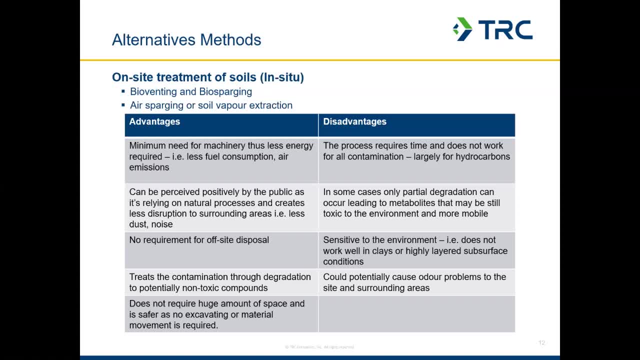 for extensive amounts of equipment and machinery. Again, it could be perceived positively by the public as is. relying on natural processes does not involve any kind of excavation of material, which would lead to less disruption to surrounding areas and so less dust and noise as well. There's no requirement for any off-site. 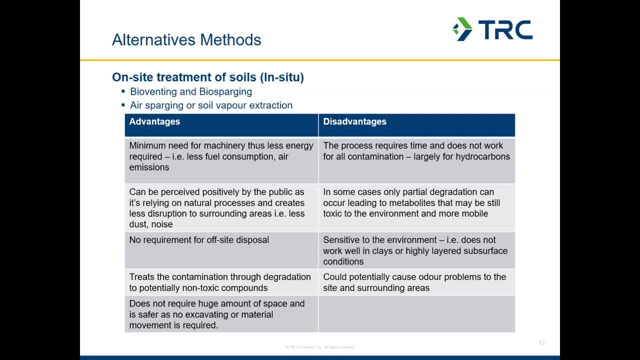 disposals saves on landfill use. Again, this method will actually treat the contamination and hopefully break down the pollution. So again, these are the benefits of ex situ soil vapour extraction: break down the toxic compounds to non-toxic compounds and it does not require a huge. 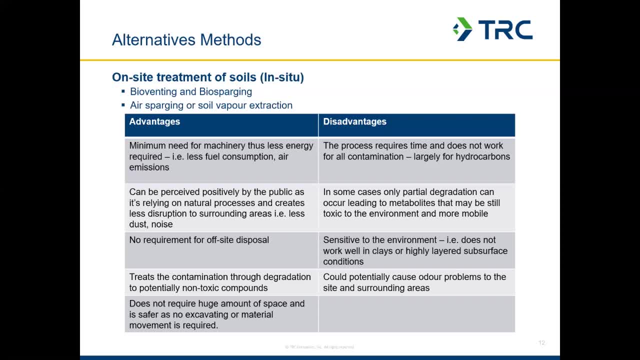 amount of space and, again, it's a safer process as you're not having to excavate any material out of the ground. Again, there are disadvantages to this method: The amount of, so this method would also take a considerable amount of time, so that's something to consider. plus, it's not suitable for all kinds of contamination. 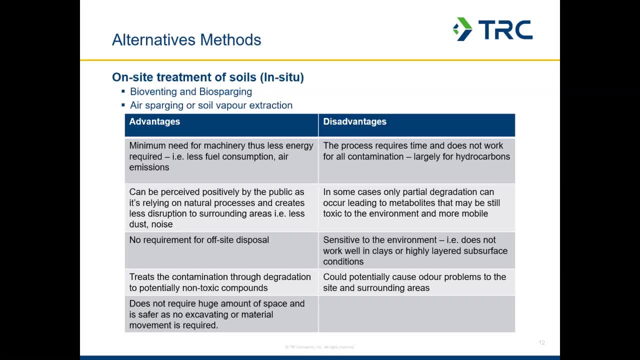 It can also potentially cause odour problems to both the site and the surrounding areas. so again you need to consider odour control measures. It may require more monitoring on site again to determine whether the process is happening. so this could add more costs and again it's a 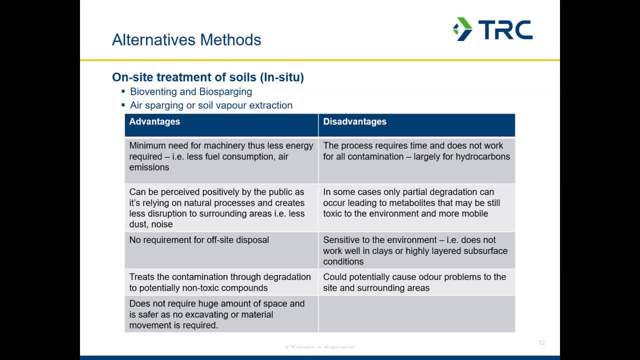 highly. it's a method. it's a method that's highly sensitive to environment pollution. So, as you can see, there is no one method that has all the positives with no negatives. The important message here is to strike the right balance and to consider all available options. 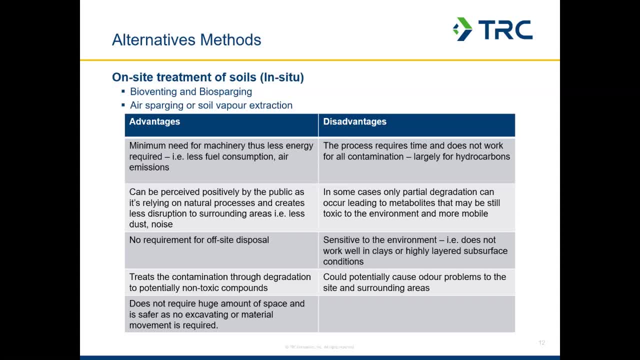 before selecting the most appropriate method. As previously discussed, there are many things to consider besides the contamination itself, and every site is different and presents its own challenges. As mentioned earlier on in the presentation, there are many things to consider besides the contamination itself, and every site is different and presents its own challenges. 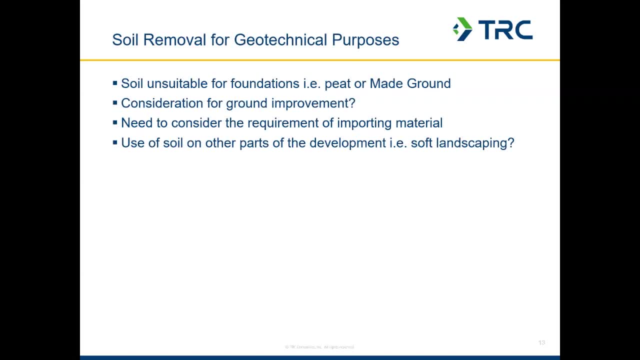 As mentioned earlier on in the presentation, there are situations where soils are environmentally suitable but not geotechnically suitable for foundations, so I just want to touch on this a little bit. When that occurs, you could have a soil that are perfectly fine environmentally. that has. 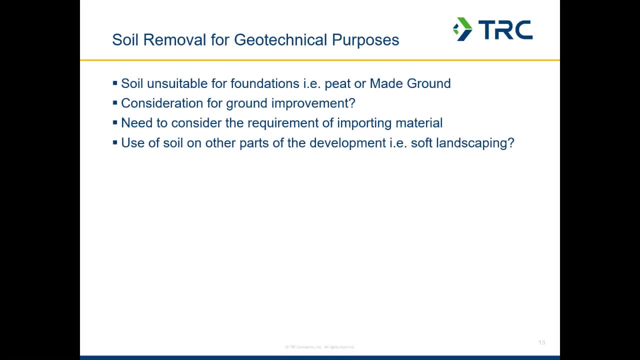 to be removed and disposed of off-site as it's not suitable for founding on, and this would again lead to significant haulage and result in all the issues that I've previously discussed. Considerations should be made with regards to whether it's necessary to excavate and remove. 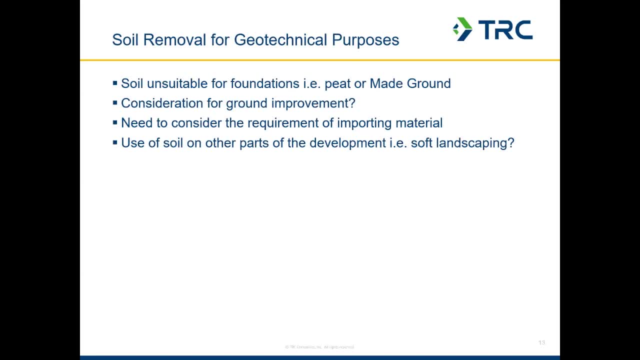 these soils from site. Could the client consider ground improvement as an option? It could be that the cost of ground improvement versus soil disposal would be fairly comparable. However, with ground improvement you would also need to consider the the need to import materials to do the ground improvement and again this could lead to higher. 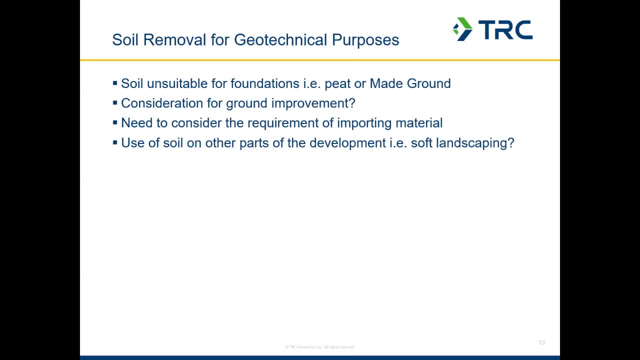 costs and again you'll be transporting more materials to the site, which is not the most sustainable way of doing things. Could the client consider using the material removed on other parts of the development, such as in soft landscape areas, if deemed environmentally suitable? This would save on both disposal and import costs, so it's definitely something worth considering. 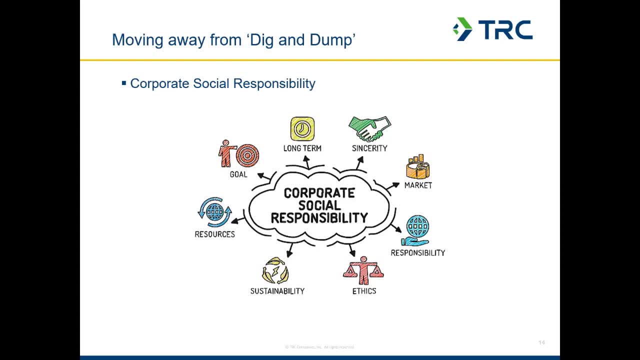 So, unfortunately, the majority of the time, remediation methodologies selected are purely driven by time constraints and costs, which makes it difficult when trying to adopt a more sustainable remediation approach. So how best can we convince clients to consider a more sustainable approach? A lot of companies have corporate social responsibilities and being seen to 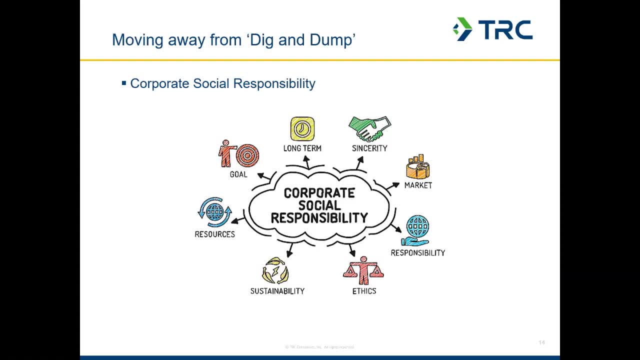 consider sustainability when remediating will demonstrate compliance to their policies and will benefit them by giving them positive public relations, as they'll be seen as doing the right thing. I also think engaging with clients early on in the process could help them see the importance of sustainability and to best inform them of the other methods that could potentially be adopted. 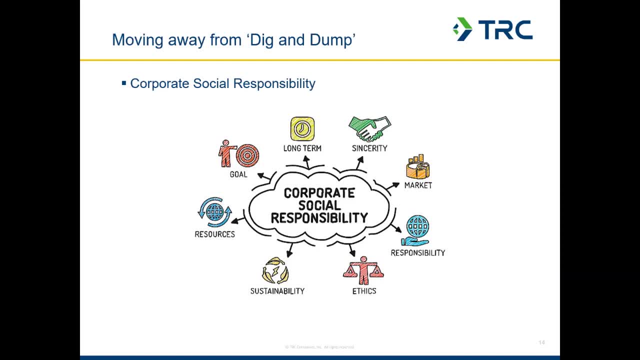 on site. I also think engaging with clients early on in the process could help them see the importance of sustainability and to best inform them of the other methods that could potentially be adopted on site would assist them developing their program of works and allow them to include time for remediation. 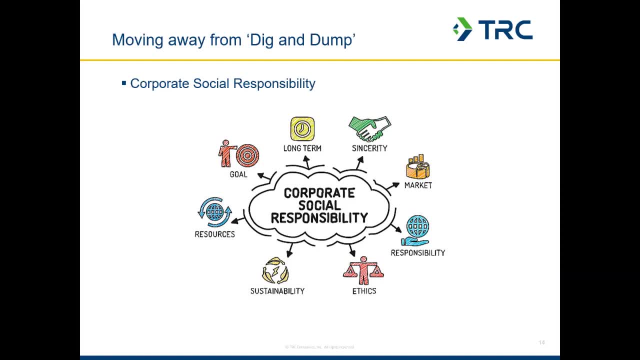 If clients can see the bigger picture, they may be more open to consider more sustainable options. It is likely that clients would be more open to more sustainable options of remediation if they are provided provide economic incentives to do so, And I think that's it. 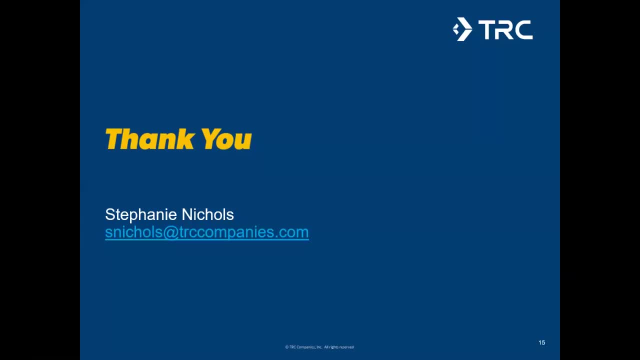 So thank you all for listening and yeah, I hope you found it informative and yeah, if anyone has any questions, Fantastic. thank you, Stephanie. that was really interesting and there have been quite a few kind of comments just for discussion and questions come in. But before we kick off, there's just one point of clarification that an attendee is seeking. 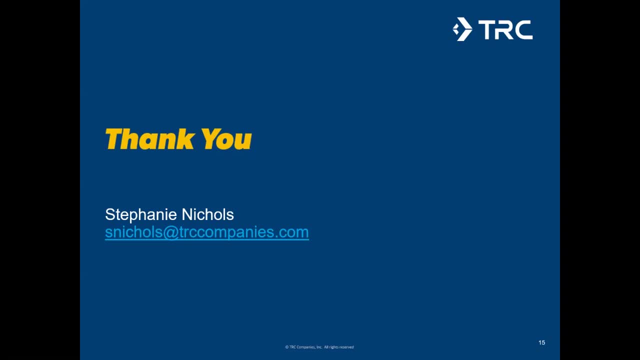 just to ask what is meant by below the footprint that you mentioned? So the building footprint, so where the building will essentially stand. Okay, fantastic, thank you. hopefully that answers the attendees questions, but if you've got any more, then do let us know. Okay, I'm going to kick off with the first one to say is one approach to increasing. 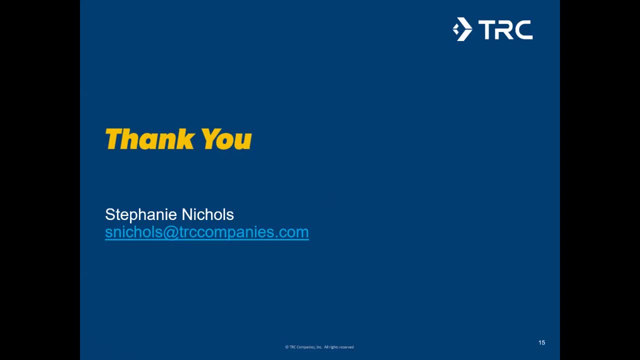 the consideration of, to increase the consideration of non-dig and dump approaches, to raise the weighting that sustainability gets within the remediation appraisal. Yeah, that would be something that could be considered because I think at the moment remediation options appraisals might not necessarily be carried out. you know from my experience. a lot of the time, you know we don't. 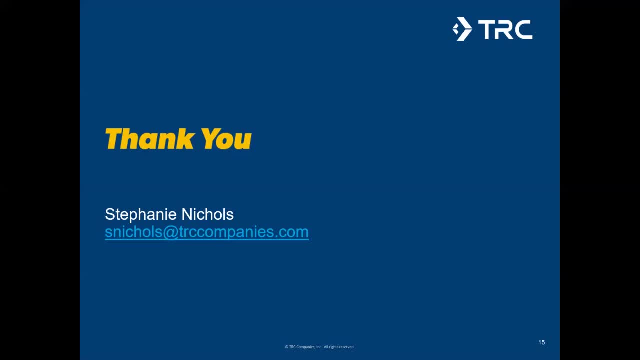 really have the time to actually do a proper remediation options appraisal due to sort of program limitations and I think, and also there are times where people do not consider sustainability when doing their appraisal. So I think that's something that we need to think about as well. 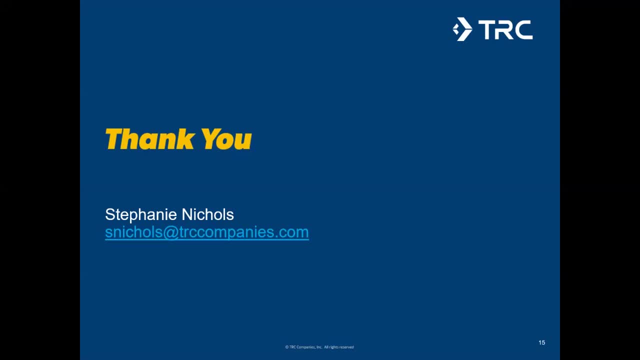 Yeah, I think it's definitely something that should rank higher when carrying this out. I mean, there's like I said before, there's no one correct way of doing it. I definitely think it's worth looking at the SURF UK framework for a bit more guidance on it, and I find that 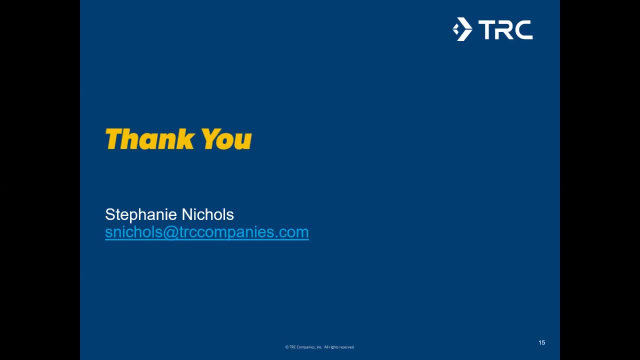 quite useful and it's available on the Clare website. Okay, that's really useful. somebody has asked whether it is if scoring or weighting is purely subjective or if they're just doing it to their own benefit. The answer would be yes if they're doing it to their own benefit, and that's what we need to do. 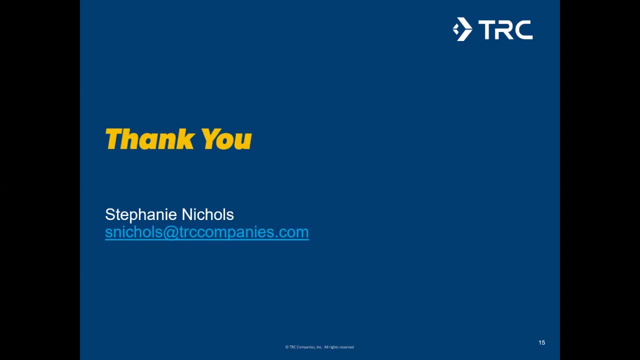 there is uk guidance. so, yeah, you've mentioned it's the only yeah, the yeah, the class. sorry on claire. they, they provide. um, there's a lot of resources on there regarding this method and there's a spreadsheet on there that's been developed by urs that can, that can sort of give. 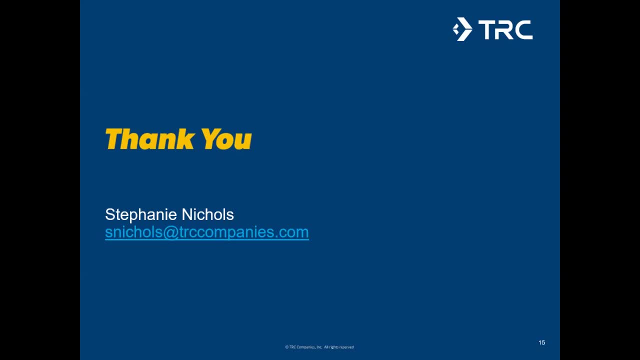 you some guidance on how to carry it out. so it does have a sort of three-tiered approach where it starts with qualitative, then it goes to semi-quantitative and then it's a quantitative assessment. but yeah, there is good guidance on there, so it's definitely worth looking at. 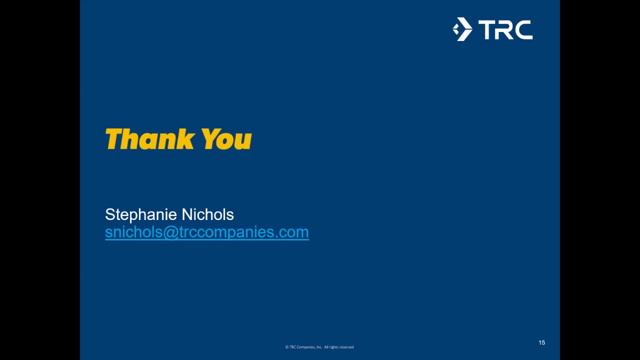 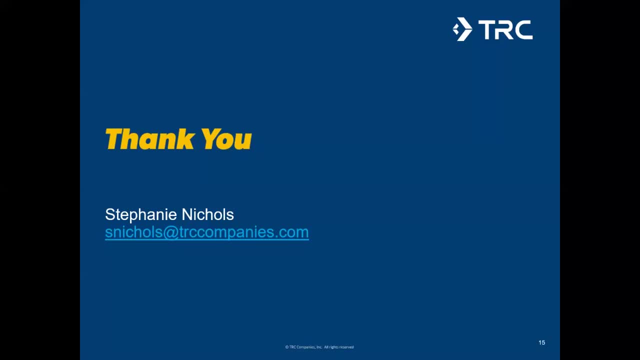 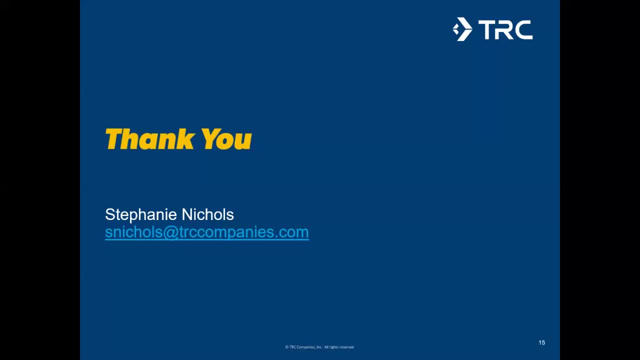 and they'll be able to tell you early on whether something is feasible or not. um, so, yeah, i do. yeah, i agree, i think that does. yeah, that is something that, um, yeah, we should consider, or clients should consider, sure, okay, um, a question around, um with the new lcrm soon to be adopted by all consultants. 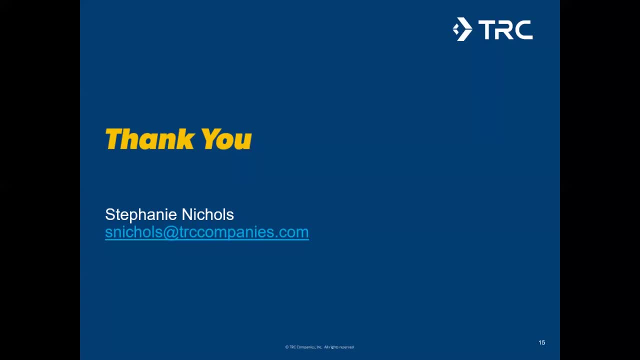 would there be a necessity to provide some sort of guidance or directive with regards to the soil remediation technology and costs that aid the development of the stage two options- appraisals, reporting, or which can be the knowledge of key stakeholders? oh sorry, could you repeat that again? that's a quite a long question. yeah, with the new lcrm. 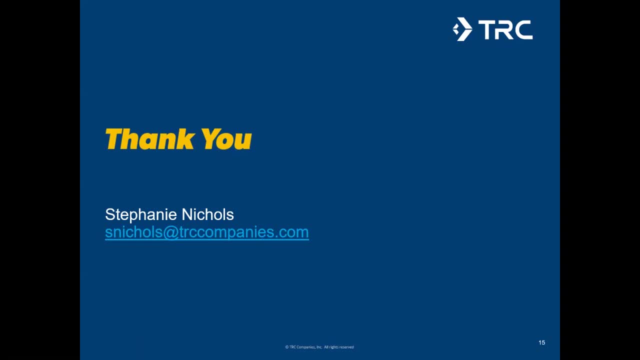 soon to be adopted by all consultants, um, with regards to the soil remediation technology and costs to aid the development of the stage two, options which can of appraisal, reporting on, which can benefit the knowledge of key stakeholders. oh you, would it be necessary to provide some sort of guidance, um to this group? um, yeah, i think it would. 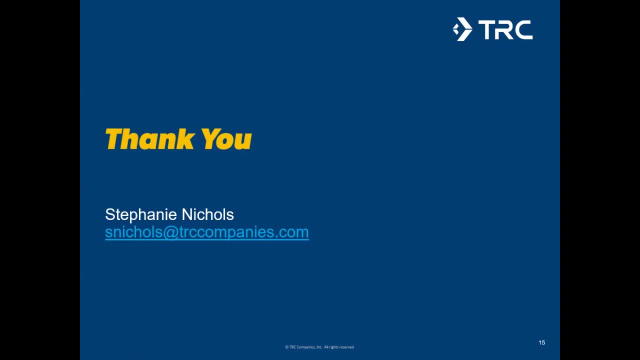 be? um, i'm not sort of- yeah, i'm not sort of that sort of clued up on it right now, so i'm not really able to provide too much um on that. sure, okay, no, that's absolutely fine. um, do you find that regulatory requirements put developers off from non-dig and dump remediation? 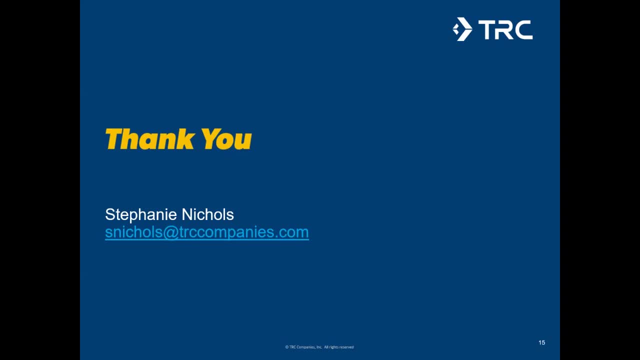 yeah, yeah, i, i i do sometimes um. i mean i think it's from my experience- it's always worth engaging with uh regulators and um early on um. i find, yeah, there is an element of sort of developers being being put off by um going with any other options, because i think you know they know that by doing dig and dump, that essentially um, it's the most important thing to do so i think it's always worth engaging with regulators and early on um. i find, yeah, there is an element of sort of developers being being put off by um going with any other options, because i think you know they know that by doing dig and dump, that essentially um, it's the most important thing to do. so i think it's always worth engaging with regulators and early on um. i find, yeah, there is an element of sort of developers being being put off by um going with any other options, because i think you know they know that by doing dig and dump, that essentially um, it's the most important thing to do. so i think it's always worth engaging with regulators and early on um. i find, yeah, there is an element of sort of developers being 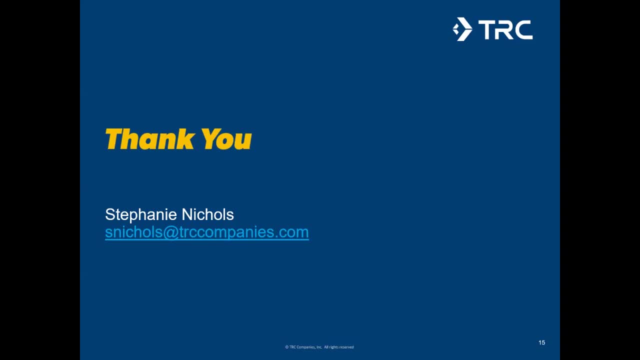 straightforward way of treating the problem and it is an accepted way of of dealing with contaminated land. but um, i i think if you were to engage with regulators early on it's. i think that definitely helps and from my experience i'm pretty sure the regulators would appreciate it. and you know i. 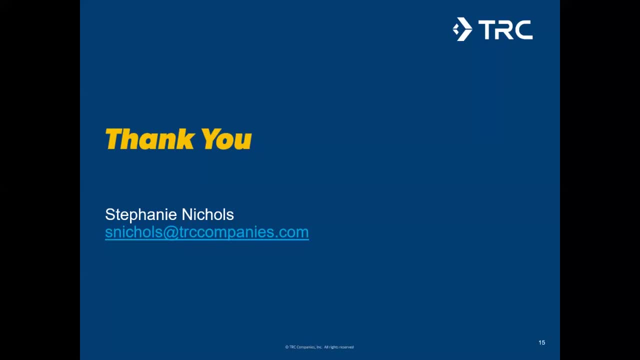 think there is just an overall goal: to be more sustainable. so i think it would you know if you were to engage with them early and explain what you- you know- hoping to achieve. i, i don't, i'd like to think it does. it shouldn't put um developers off. but yeah, i i, from my experience, it does tend. 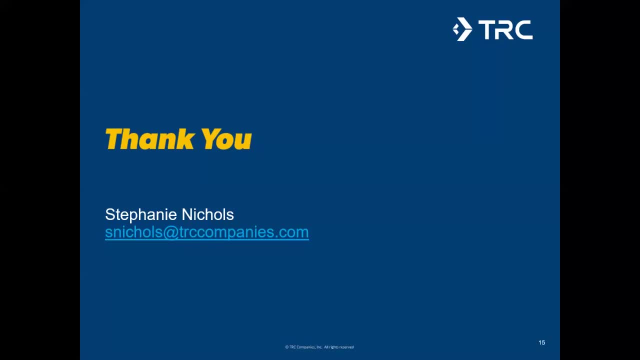 to be. they just want to get the problem resolved quickly, um, so yeah, they're just happy to go down the dig and dump route to avoid too much, too much back and forth. essentially, um, okay, um, do you are there any effective treatments for persistent organic contaminants of heavy metals and for heavy metals you know? oh, um, i might have to pass on that one. 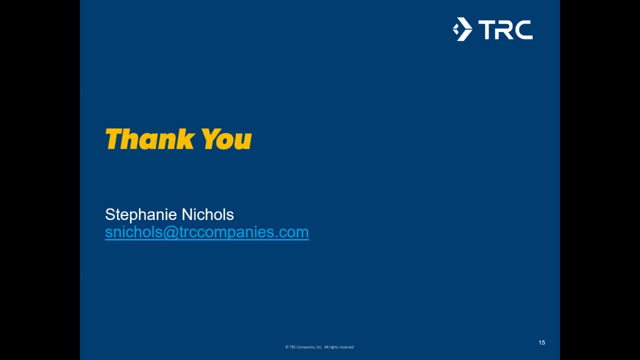 um, yeah, sorry, no, no, that's absolutely fine. um, another thing is: some researchers have shown that the efficiency of sorption, absorption methods, such as the use of activated carbon and biochar in soil remediation. um, how soon do you think that this will be seen as a 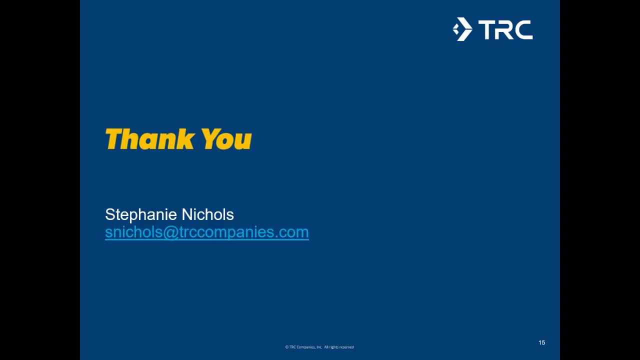 method in uk industry? um, or do you think it would be at all? i, i think, as there's a push to sort of be become more sustainable, um, in all your sort of remediation technologies, i, i do think that it's, it's something that you know that people will try and move away. 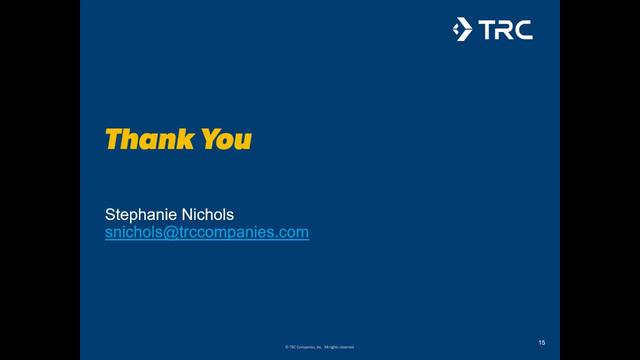 from the, from the dig and dump method, and adopt sort of more um, sustainable options like the one you just mentioned and, um, i think, um, yeah, i just think, yeah, i think we were, we are, you know, from what i can tell, i think we are moving away from that and moving to more innovative methods. so 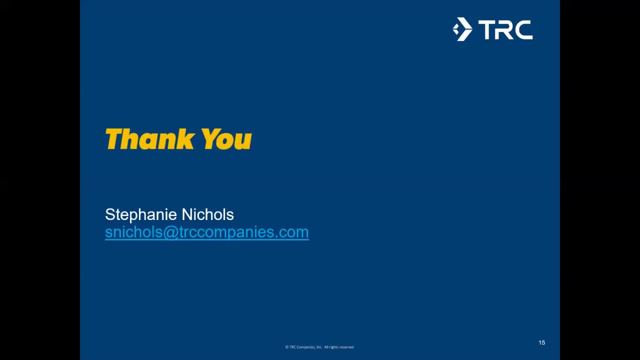 i think it's all down to you know, research and and sort of you know projects that have demonstrated that this is, that this works. and i think the more sort of research we have or the more case studies we have to demonstrate that these methods are, you know, are working, i think 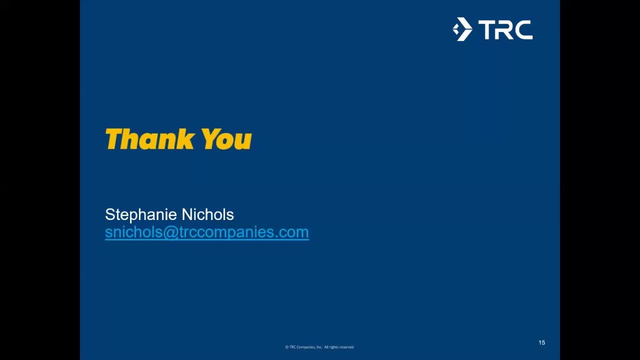 you know we stand a better chance of moving away from dig and dump and using um methods like that to to remediate. okay, brilliant. well, there's one question about a slide that you had up earlier on and where some of the data was quite quite small and to read: oh yeah. 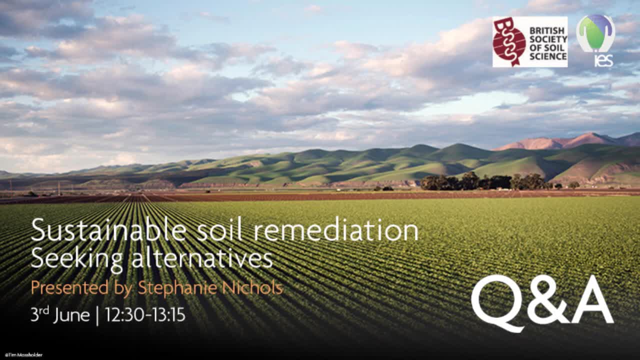 sorry, this may, this may, this question may refer back to that. so do you have some indicative figures on the amount of remediation that happens currently in the uk? um, and if, if there's any kind of correlation with particular regions? oh, i don't have any. no, i don't. i think i. i think you were, it was probably the slide where i had the 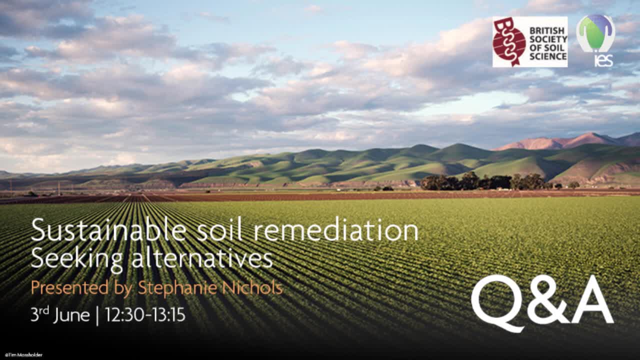 pie chart showing um the amount of waste soils that are generated um every year. i think that might have been the slide, but uh, i think if you look on, i think i got this information from um defra. there is a document um. i mean i can send it to you later. 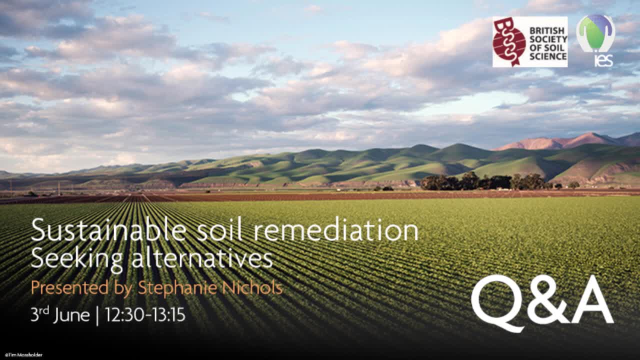 rihanna if you want to share it. that has quite good statistics there, okay, um, yeah, um, also one, one question: is there kind of a barrier around understanding with developers sometimes that they understand dig and dump quite clearly, whereas anything more technical may be perceived slightly more risky or, um, unfamiliar is that? is that something that you overcome? yeah, i mean from. 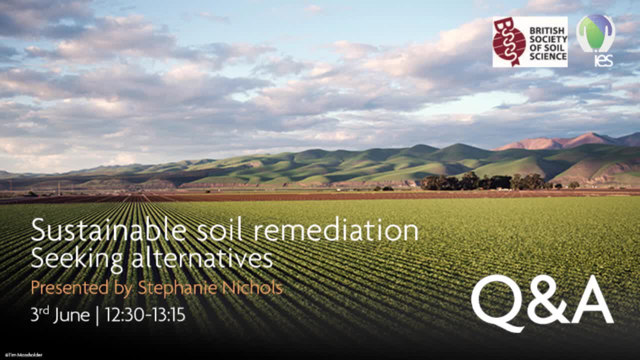 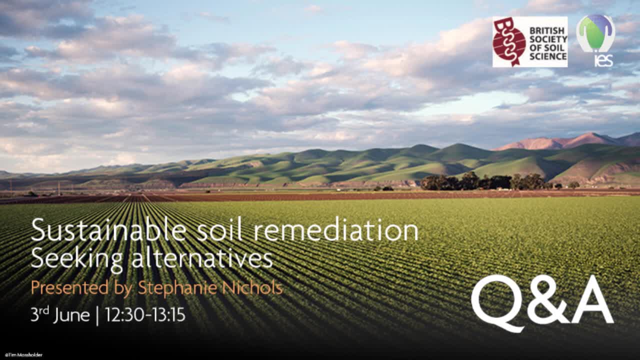 i think there are times where you, if it gets a bit too technical or, you know, for example, with bioremediation i mentioned, there are times where you you know there are risks to it, where, um, you know, contaminants may not sort of degrade completely and you only get partial degradation. 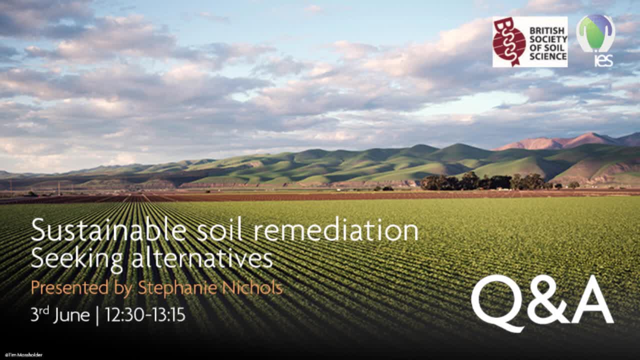 that could lead to metabolites that are sort of more mobile and migrate off-site or are actually more toxic. i think that aspect of it would make a developer more nervous, whereas with dig and dump, you know, you're sort of guaranteed to essentially remove the, you know, remove sort of the majority. 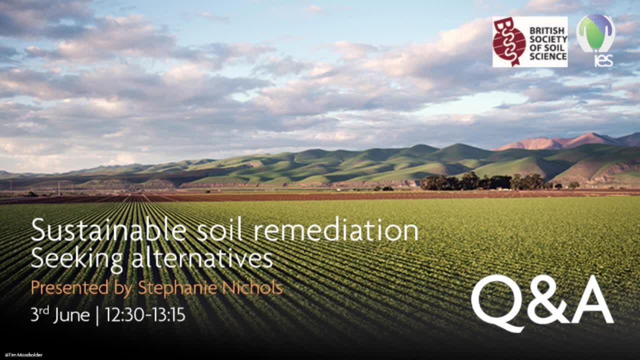 of the contamination. i think, yeah, i think it's all down to the risk and with developers to have such- you know- clients that i work for have such short build times in their programs that, um, if you try and sort of suggest anything, that's a bit more like sort of outside the realms of dig and dump. 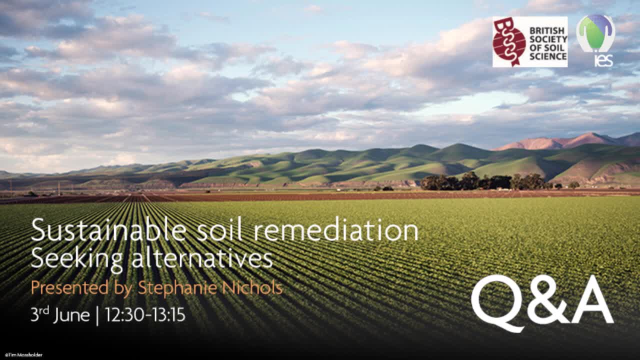 they do get a bit more nervous. so maybe it is a way you know, maybe we as consultants need to try and educate them more or sort of find a way of explaining things a bit more straightforward and better for them, because a lot of the time you kind of issue reports to clients and they 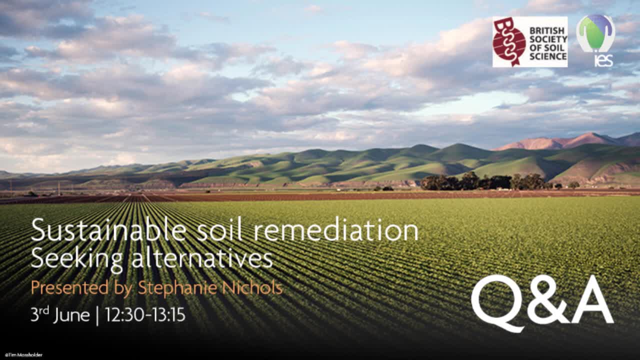 don't really sort of read into the whole technical aspect of it and they just want like a straightforward answer. and yeah, i think there is definitely a barrier, um, barrier there. okay, that's interesting, thank you, um. another one is: there seems to be kind of a current focus on the use of bioremediation, and how can we use bioremediation to help people? 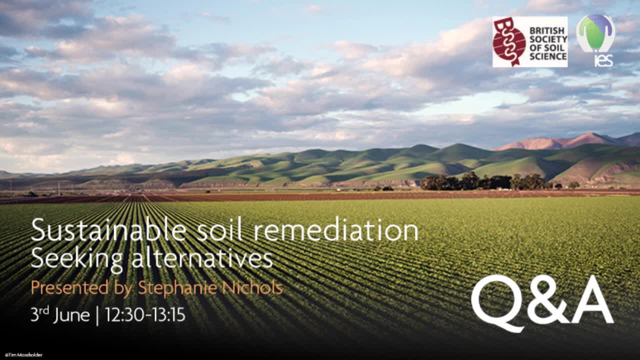 around cost and time savings. however, considering that topsoil resource is fairly finite, do you think the developers should place more emphasis on soil reuse as far as possible? um, yeah, definitely i think. um, you know, i, i've you know, i've worked with clients where they are. 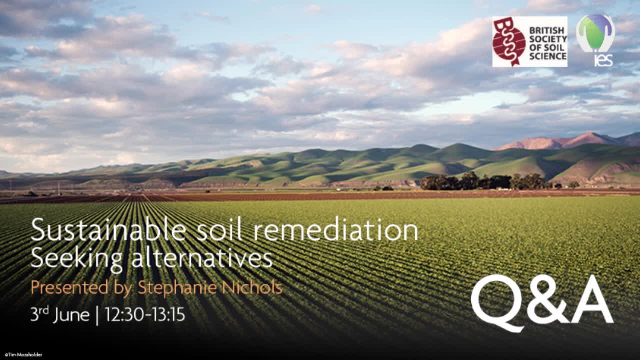 trying to. you know where you've got a site that might have a sort of a layer of topsoil on top and they are keen to, you know, to save on costs for importing, you know, clean topsoil, which is expensive. um, you know, i have worked with clients that are keen to, you know, try and reuse. 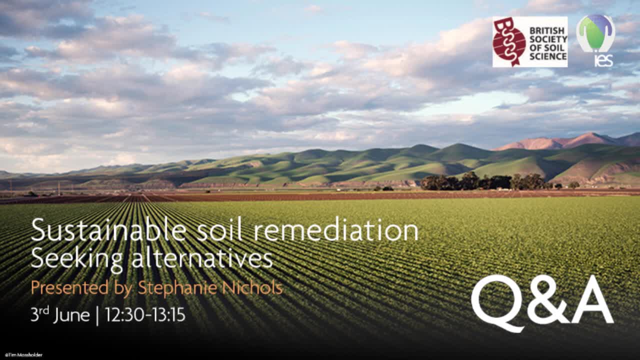 the material on site. it benefits them because it saves on costs. um, so, yeah, yeah, i think so. um, okay, um, and a question around um kind of the process really is: are there any specific places or areas where we- we as kind of professionals- can remove the soil from and then transfer it to our field, if you're in that? 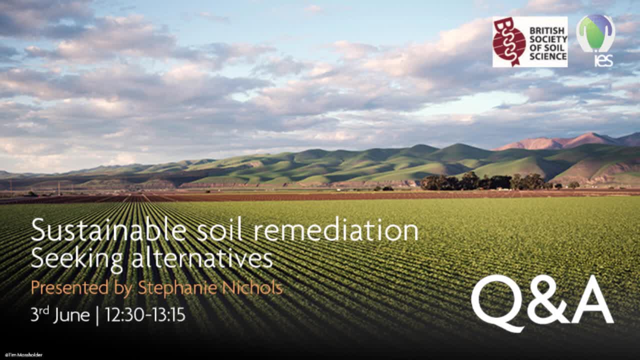 situation. so is that to do with sort of material, the movement, movement like material? i mean, yeah, there is, you know, you've got the sort of um you can have. you know material um management plans, if you've got material on a site that might not be deemed suitable for your site but can be used. 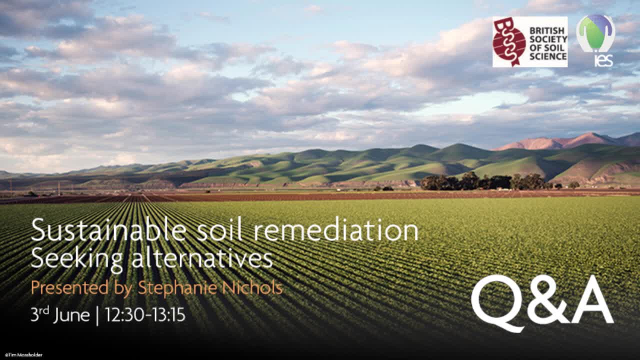 on another site. there are ways that you can, you know can- put that in place. you just need to, you know, do a materials management plan, essentially, and and make sure that you know all the appropriate sort of paperwork and exemptions, if required, are put in place. but yeah, there, you know, i've, i've. 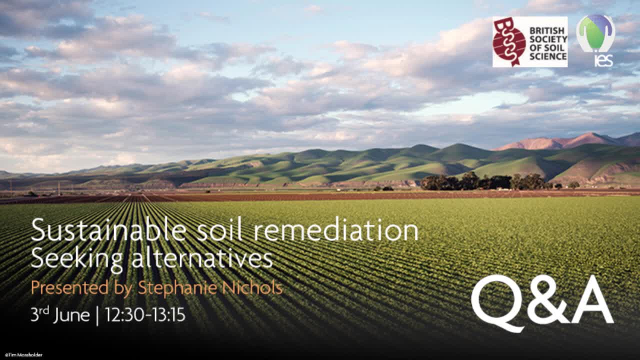 worked on sites where the materials um on the site isn't suitable for the site itself. but if you want um but then you know there's another site that would happily, you know, receive it and it is suitable for them, then yeah, that's definitely, that's definitely something that should be considered. 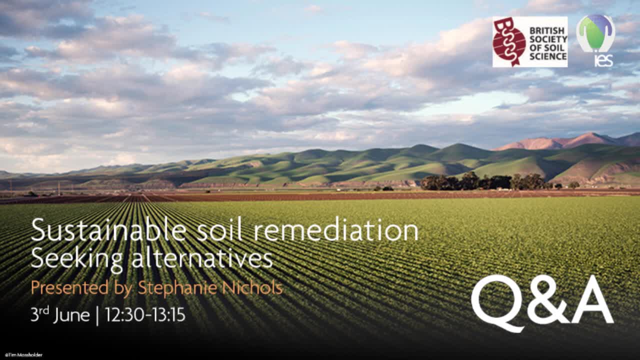 okay, thank you. and how do consultants generally keep up with scientific advancement related to soil remediation technologies? is there a kind of a good site or is there a kind of area? i think it's just. i mean, um, from my own experience i i sort of attend a lot of you know. 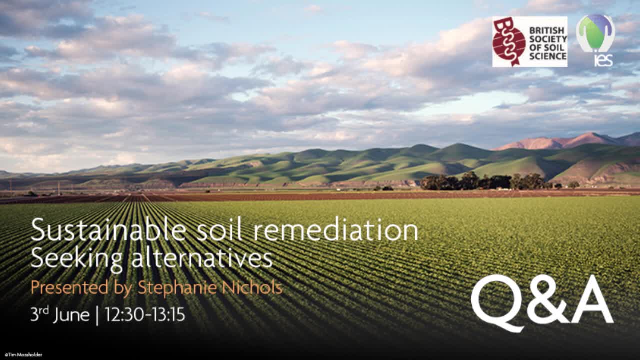 there's a lot of sort of webinars out there on on um soil remediation, um various organizations do a lot of them, um attending sort of conferences. i think, yeah, it's just. i mean, it's all just part of your cpd. i think, just making time to to. 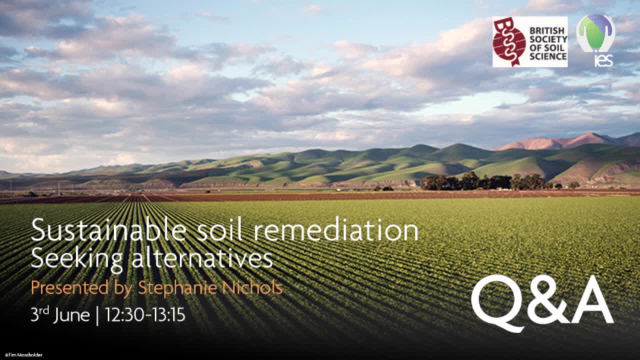 sort of sign up and attend um, you know, a lot of these webinars are free. there are a lot of you know um companies, uh that sort of remediation companies that offer free webinars on various remediation technologies, and i think that's a really good resource. 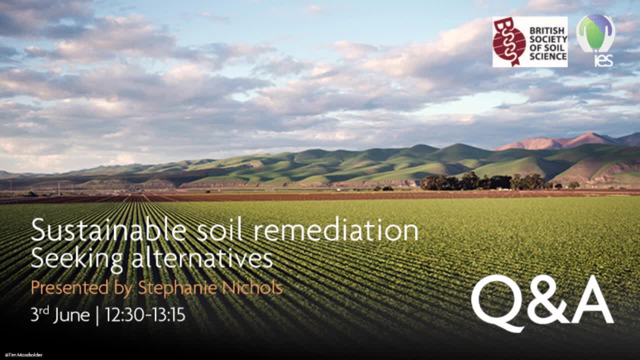 to use um to just educate yourself and sort of help you can, you know, consider these. you know potential options for sites that you might be working on? yeah, definitely, i agree. i think that, currently as well, there's a wealth of online cpd opportunities that the majority of which are free, and, yeah, those wherever you can and if you are ies members. 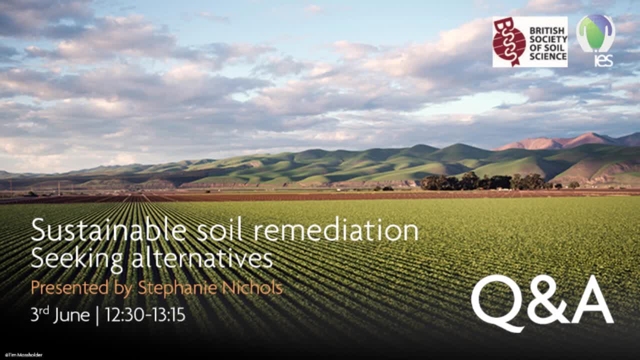 we try and do our best to circulate things that we come across and through various linkedin pages and on our website as well. so keeping abreast of those things as well um a question kind of for you. really, i think it's a bit of a curiosity about how you um work. but at the start of the 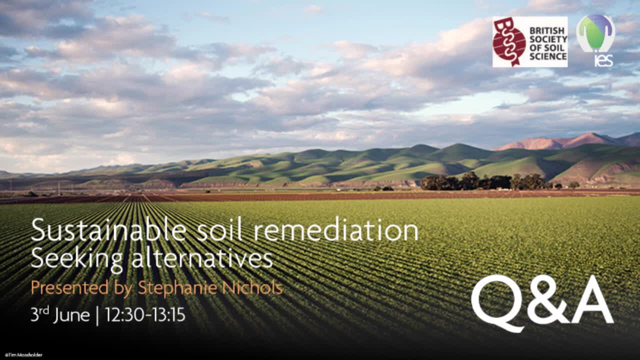 project. how do you decide which contaminants to look for considering? you can't analyze for everything- and how do you prioritize? um, well, i mean looking at the for me is looking at the site history. um, you know, if you've got a site, that's you know, that's just, you know a field for. 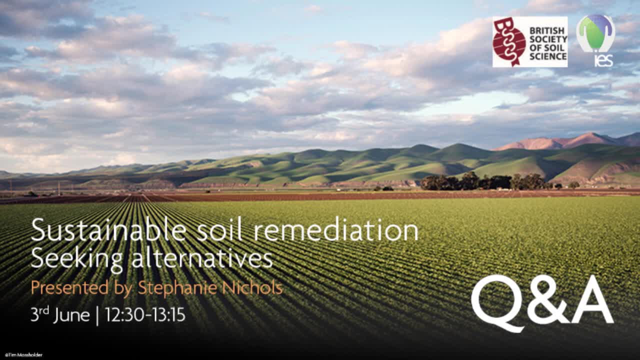 example, that's never really had much going on there. you would generally go for a like a general suite which would comprise some, you know, heavy metals and hydrocarbons, just to just to give you a general idea- um, and then obviously, if you've got um, like you know, like a gas works, you'd be looking to target contaminants. 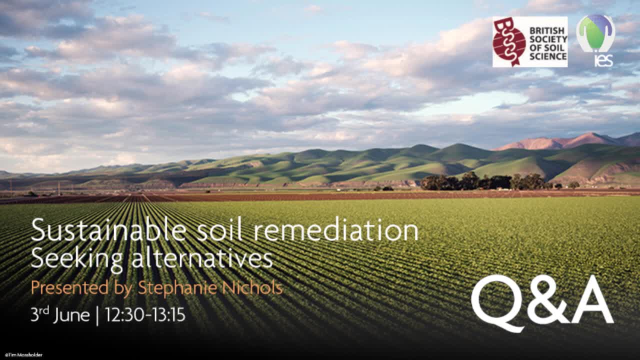 associated with a gas work. so you know, cyanides, um, ammonium, that's yeah. so it's kind of just dependent on, like phenols, you know, just dependent on site by site. so it's always so important to look at the site history, um and yeah, and any other available information the client might. 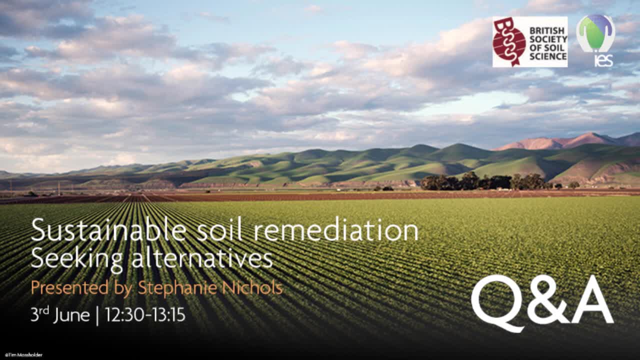 have on a site. so obviously if a phase one's been done previously, that that would be a very useful resource in helping you determine um, and it might be that you just target certain areas of the site for certain contaminants once you know. you know, for example, if you have an electricity substation. 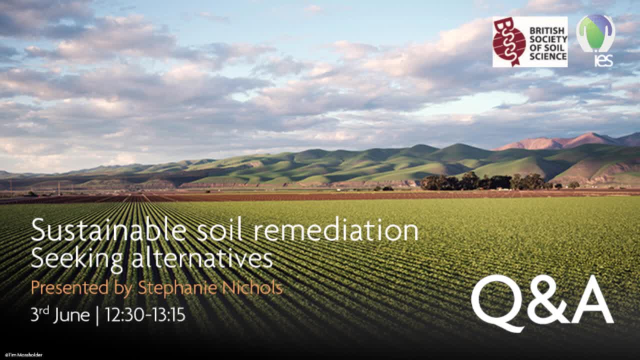 on a site you might want to um pcbs, but you know you might not. you know, if you're sort of restricted by budget, you might just do a few samples testing for that on certain parts of the site um. so yeah, it's kind of targeting the right parts of the site, um, i think that's the best way. okay, thank you, and we are running. 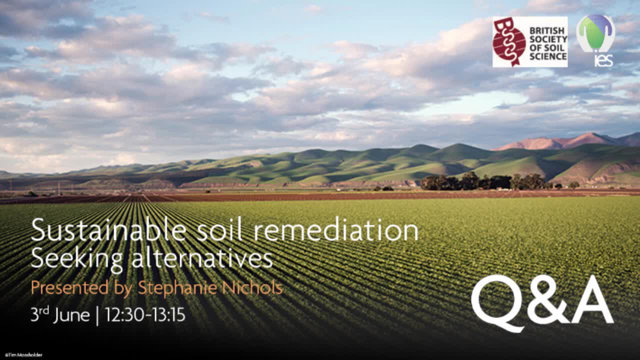 out of time, but i just want to ask you one question. it's a slightly different approach. it's just recognizing that there's an increase of environmental awareness again around the general public and within the sector are feeling feeling more pressure. do you think that um clients will start to focus on sustainability as more of a priority? 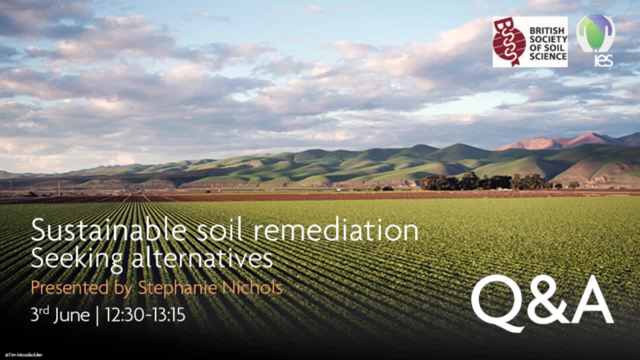 um, i, i think so, yeah, there's definitely been, uh, in the last few years, a massive increase in um people's interests in in the environment and the topic of sustainability and, like i said, mentioned in my last slide. i, you know, talk about a lot of companies having corporate social responsibilities and you know sustainability is. 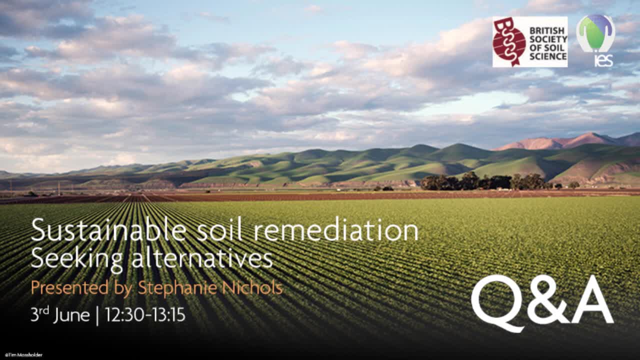 um, a big part of that. so i think, i'd like to think that a lot of companies are sort of paying a bit more attention to that and and a lot of companies do have sustainability targets. so, yeah, i'm hopeful that, um, you know, moving forward um the sort of awareness and the sort of awareness and the sort of 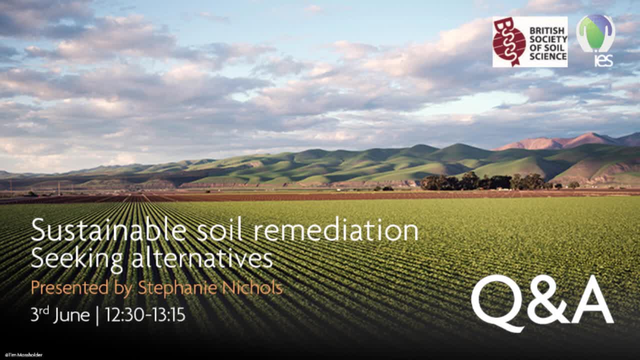 awareness will will make clients consider um more about sustainability than they have done previously. yeah, okay, brilliant, thank you. that's all the questions that we've got time for, and if there are others that are burning questions from attendees, do contact me directly and i can always put them on to steph or or answer them. so, yeah, just a huge thank you to steph for presenting. 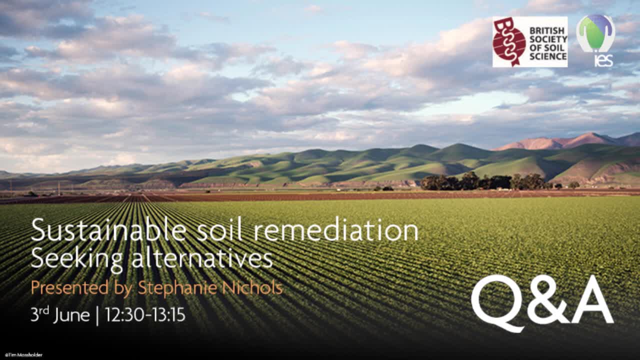 today. that was really interesting and for everybody who logged in and your questions and your questions as a cpd on the cpd tool, if you're an ies member, just log into the members area and you can do that. if you've got any problems, do contact the project office. so this webinar has been. 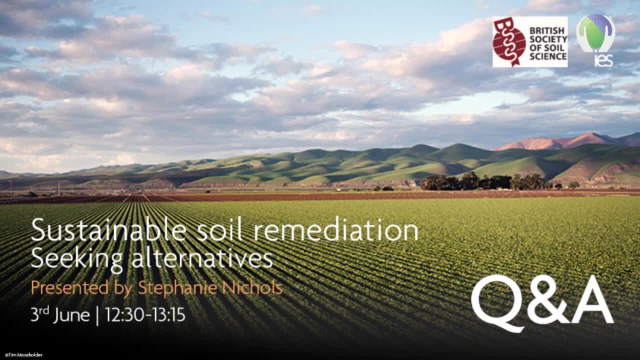 recorded and it will be made available on the ies website and the youtube channel. so do follow this and subscribe, and you'll be notified every time a new webinar is added. the next webinar is going to be on the 30th of june, on a very different subject: looking at grass seagrass restoration. 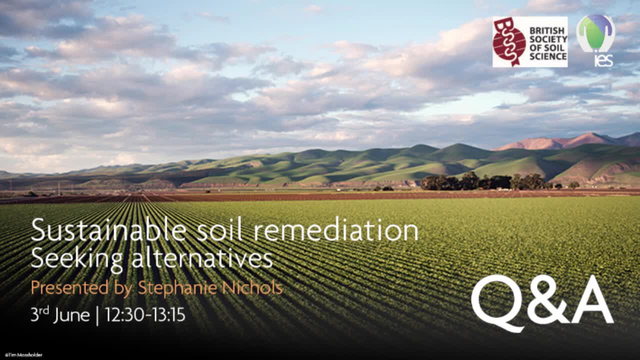 and bringing biodiversity back to the seas of the uk, and more information about that and how to register for the next webinar is on the ies website. again, that is a free opportunity. for those um professionals who did log in with a slight air quality interest. we are hosting a one-day conference online on the 22nd. 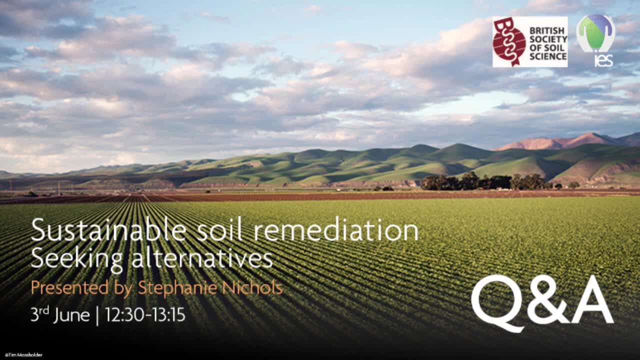 of june, which is looking at indoor air quality, and we've got speakers from bre, public health and wsp and several, several more. so details again on the ies and iqm website for those who are interested. um, but yeah, just a final thank you before we sign off to um steph and everybody.